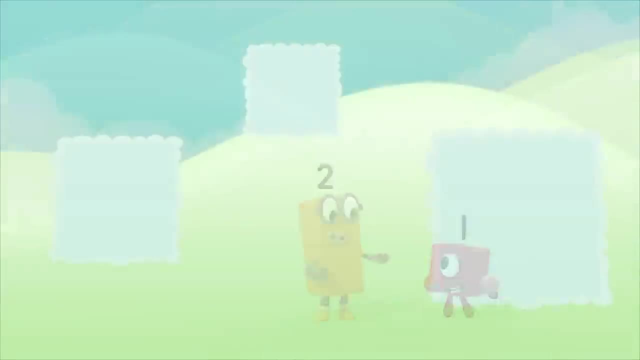 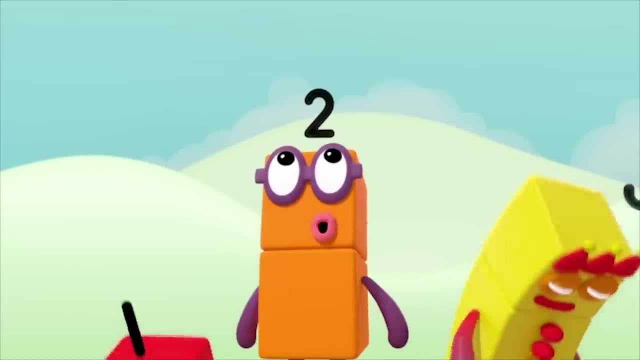 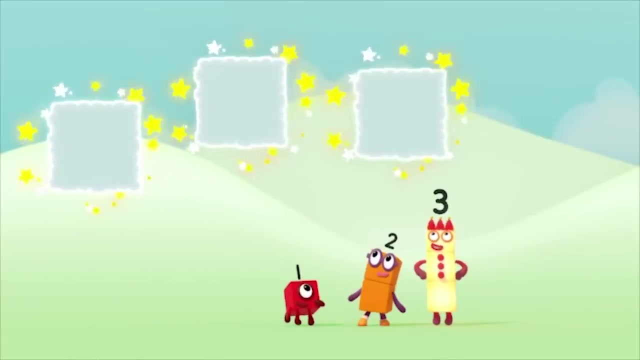 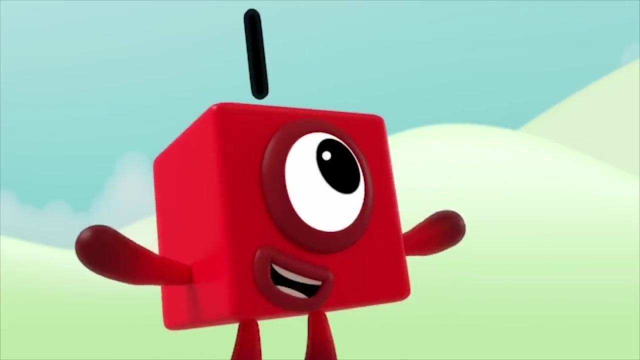 1 plus 1.. Wow, Look at the clouds. They look close enough to touch 1,, 2,, 3.. 3 square clouds And that one. We need to get rid of that one. 1, 2.. 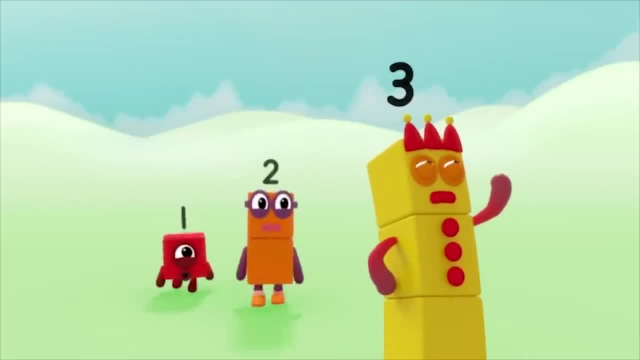 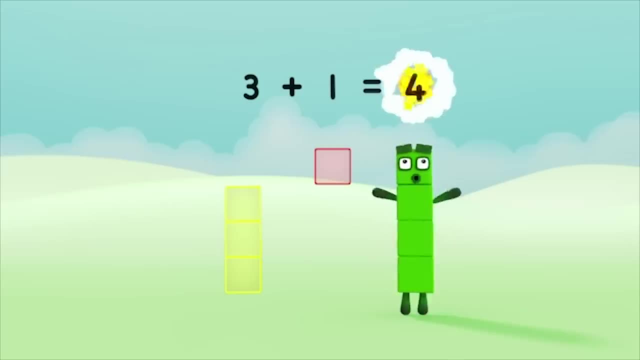 1, 2, 3.. No one's bigger than me. 3 plus 1 equals 4.. I am 4.. I'm one more. 1, 2,, 3, 4.. 4 clouds. 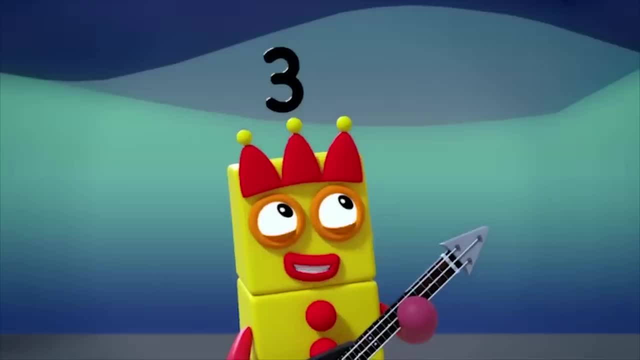 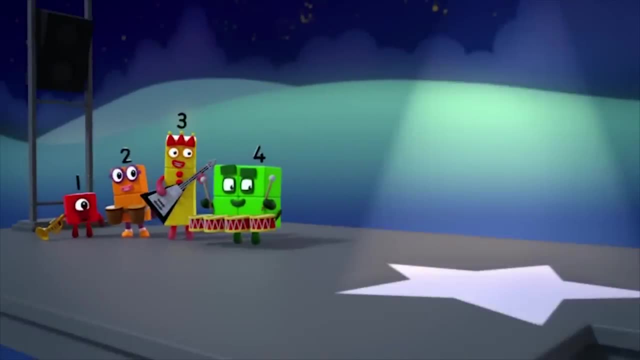 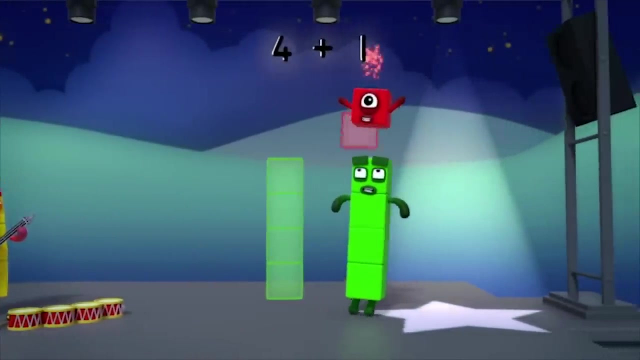 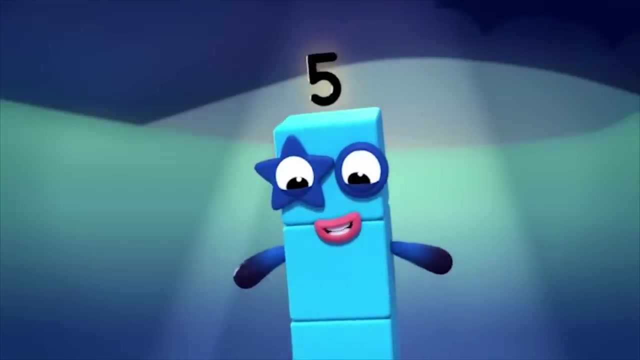 Oh, a shooting star. Make a wish. Ooh, It's star-shaped. Who's it for? It's me. Well, I'm the biggest, I'll go first. 4 plus 1 equals 5.. I am 5.. I feel so alive. 1, 2,, 3,, 4, 5.. 5 points. 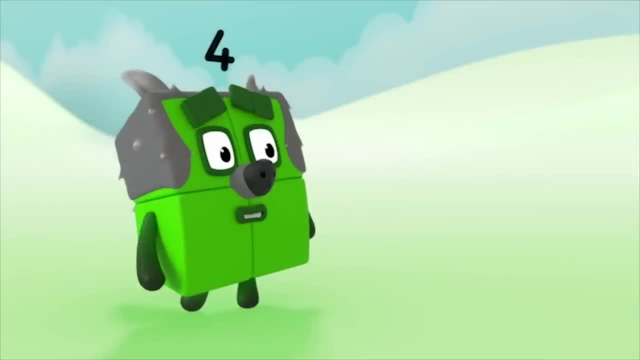 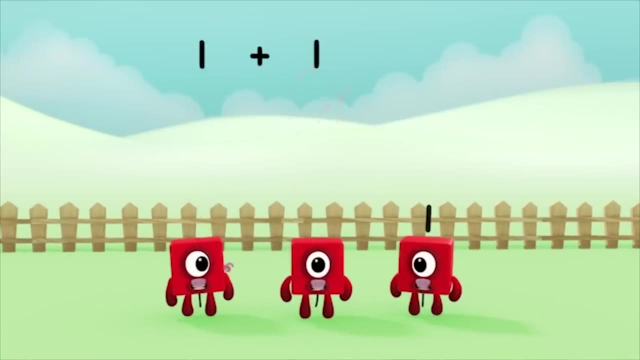 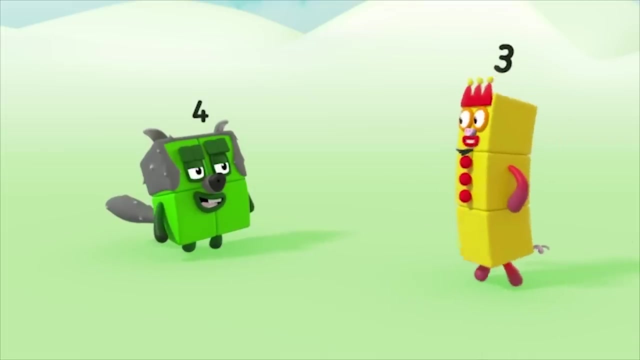 Oh, Just a little huff, dlch. Hey, 1 plus 1 plus 1 equals 3.. 4 plus 1 equals 5 plus 5.. 2 plus 1 equals 5.. See how you like it. 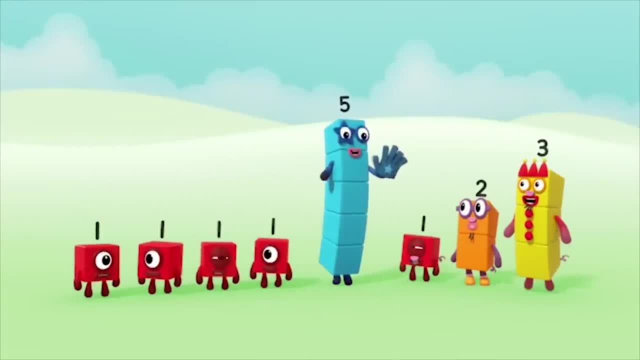 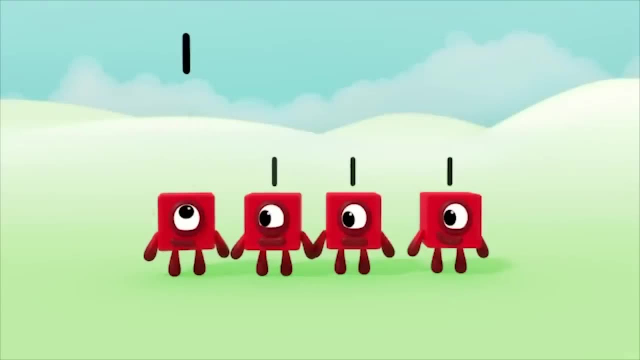 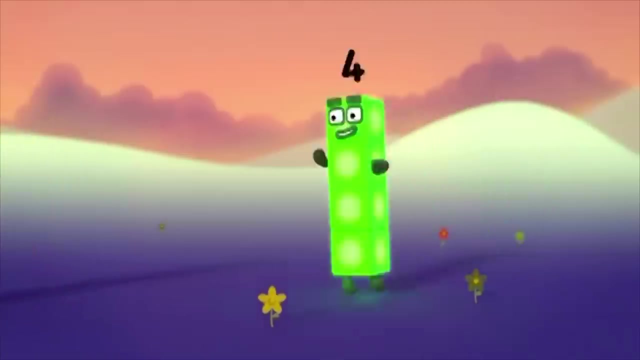 Stop, This isn't how it goes. So now you guys. The third house doesn't get blown down. But what about now? One plus one plus one plus one equals Four. I'm number four, And I am sure that I've got four blocks to play with. 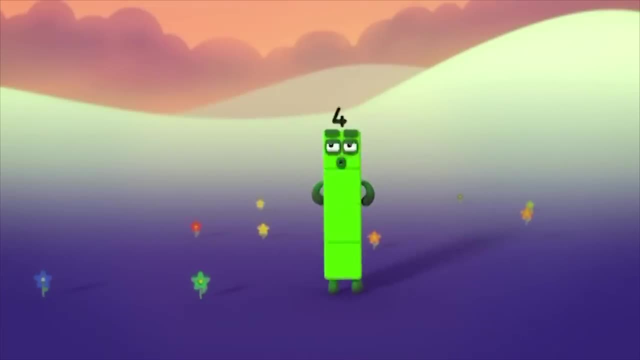 and the whole of me is four. One, two, three, four. One is a part of me and three is a part of me and the whole of me is four. Watch, I'm three and I'm a part. I'm one and I'm a part. 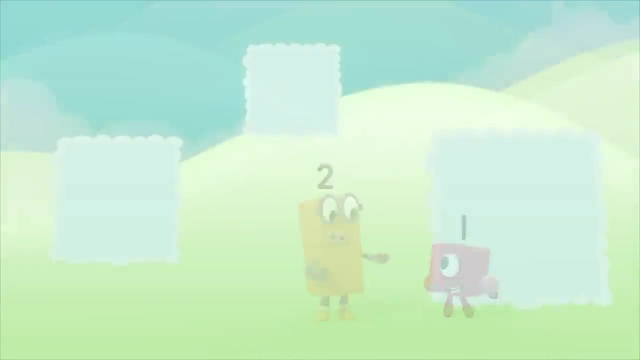 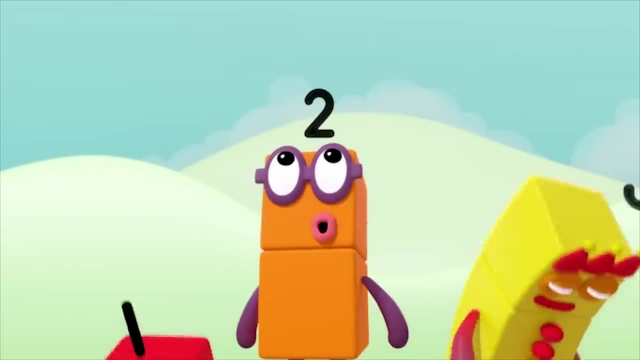 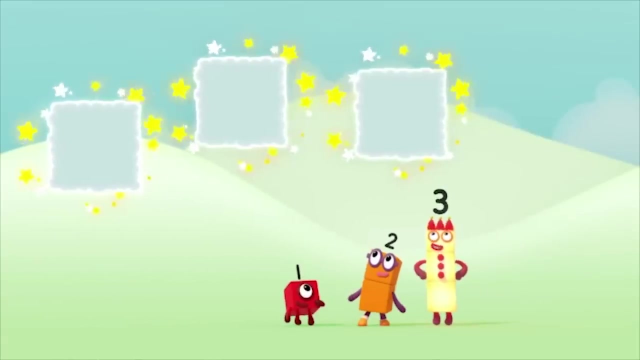 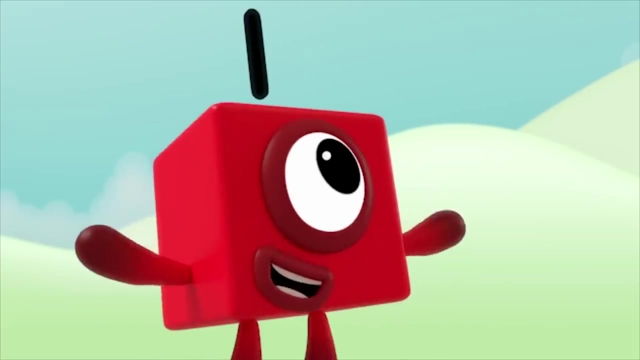 1 plus 1.. Wow, Look at the clouds. They look close enough to touch 1,, 2,, 3.. 3 square clouds And that one. We need to get rid of that one. 1, 2.. 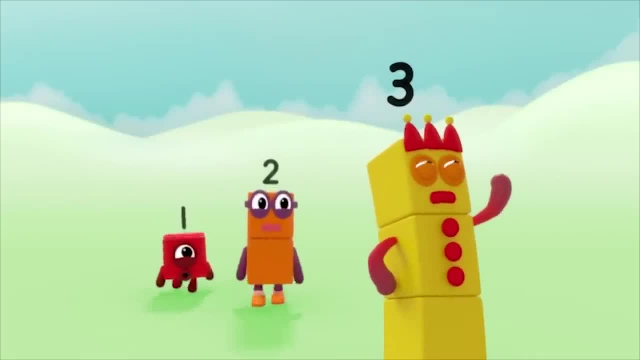 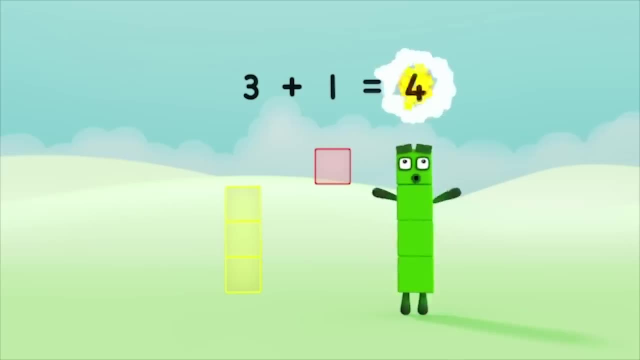 1, 2, 3.. No one's bigger than me. 3 plus 1 equals 4.. I am 4.. I'm one more. 1, 2,, 3, 4.. 4 clouds. 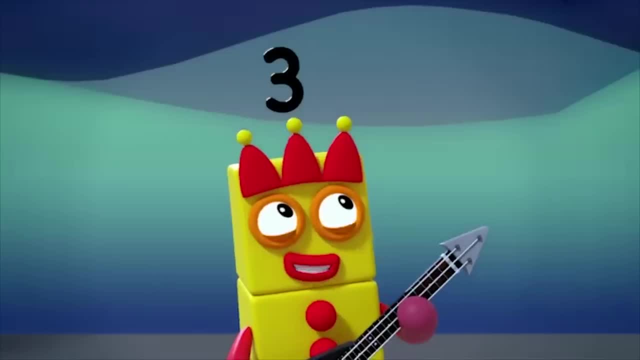 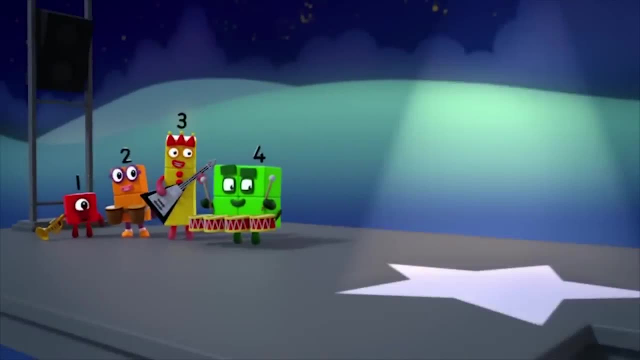 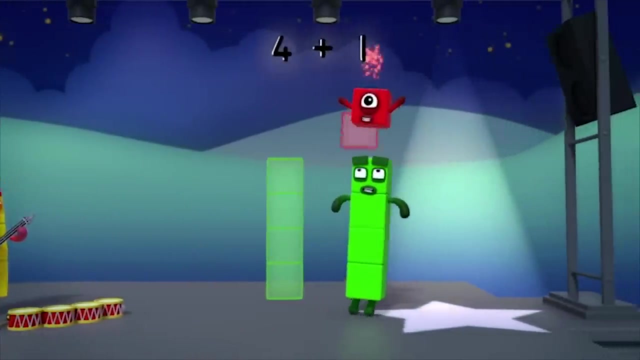 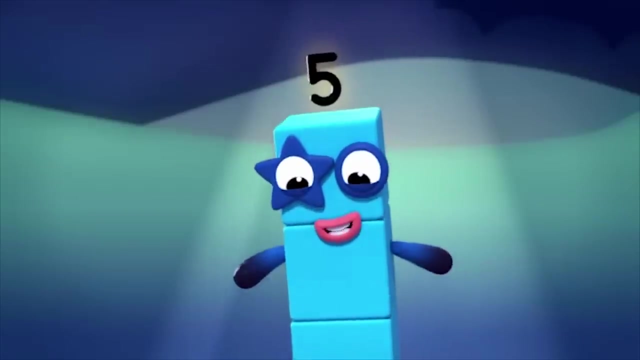 A shooting star, Make a wish. Ooh, It's star-shaped. Who's it for? It's me. Well, I'm the biggest, I'll go first. 4 plus 1 equals 5.. I am 5.. I feel so alive. 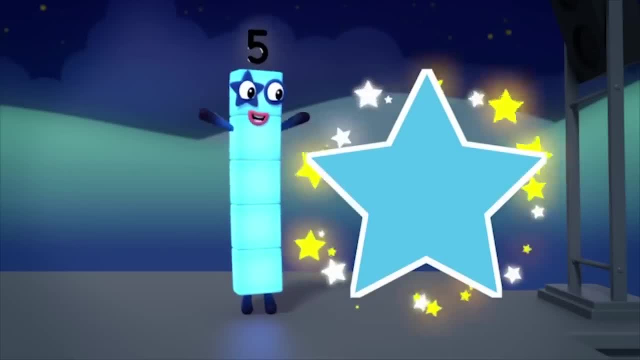 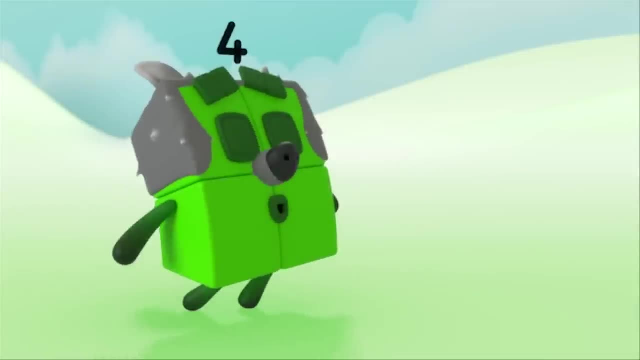 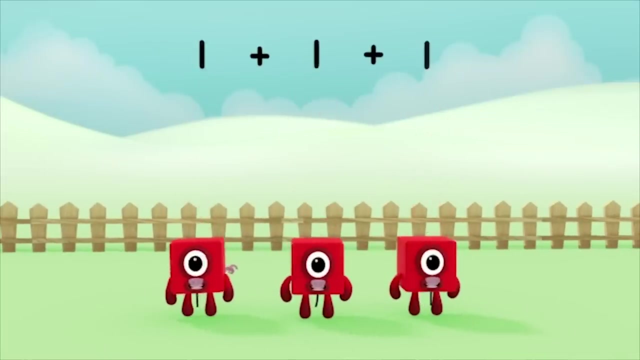 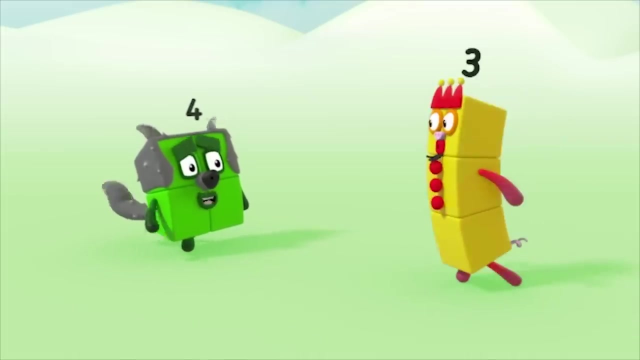 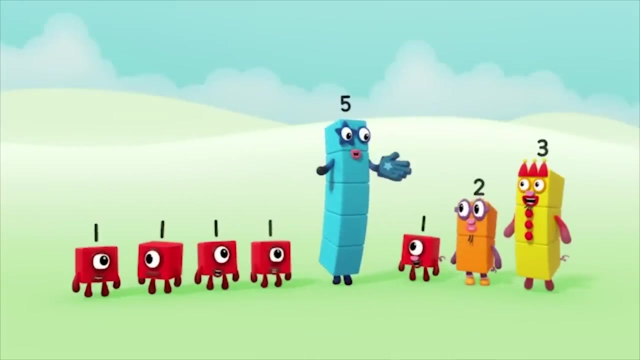 1,, 2,, 3, 4, 5.. 5 points- Oh, Just a little huff. Hey, 1 plus 1 plus 1 equals 3.. See how you like it, Stop. This isn't how the story goes. The third house doesn't get blown down. 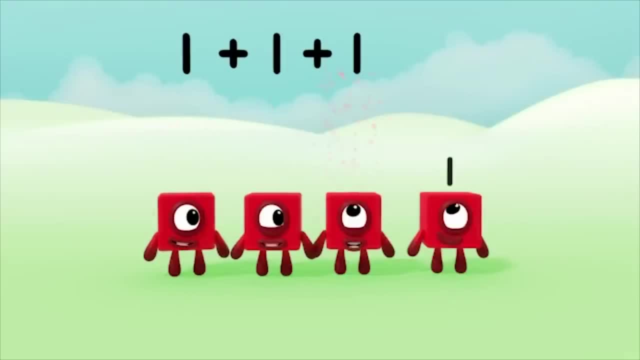 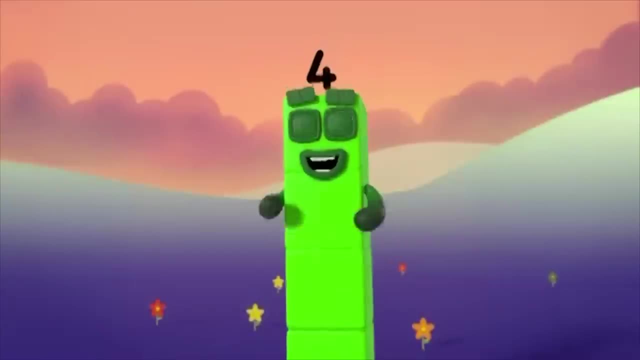 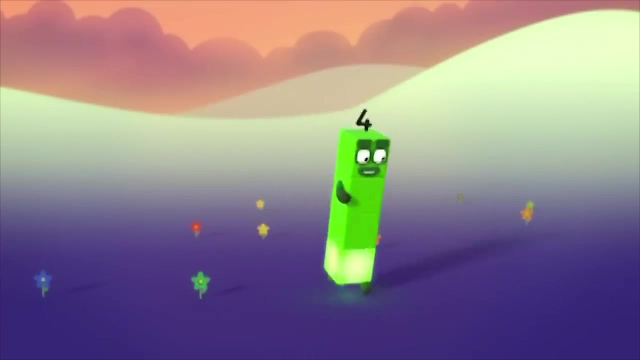 Ooh Oh, 1 plus 1 plus 1 plus 1 equals 4.. I'm number 4, and I am sure that I've got 4 blocks to play with, and the whole of me is 4.. 1,, 2,, 3,, 4.. 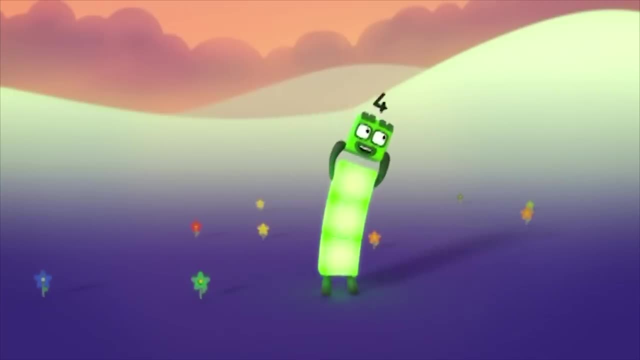 1 is a part of me and 3 is a part of me, and the whole of me is 4.. What? 3. And I'm a part, I'm one And I'm a part, And the whole of me is four. 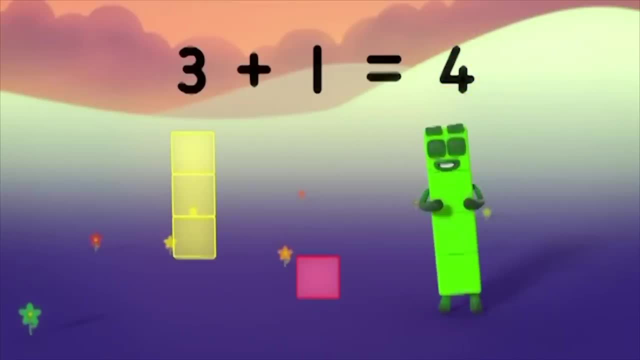 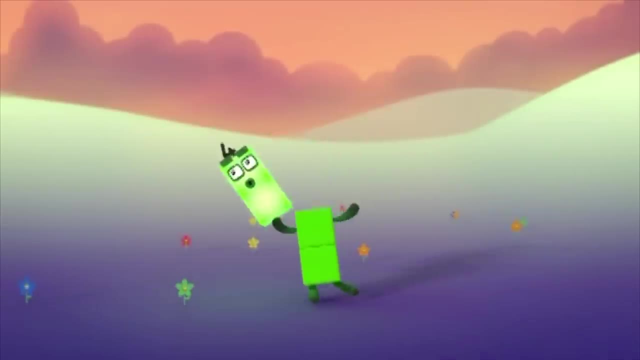 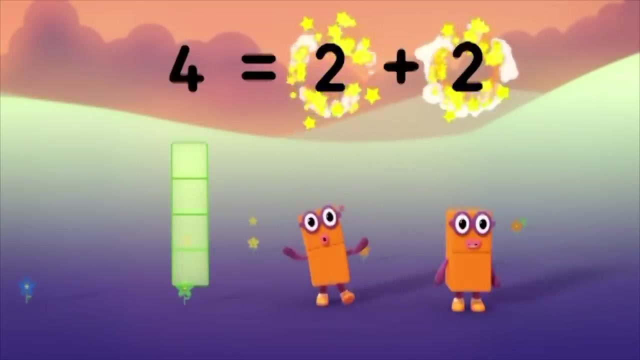 And the whole of me is four. Now here is something more that's different from before. Two is a part of me, and two is a part of me, and the whole of me is four. Watch, I'm two and I'm a part. I'm two and I'm a part. 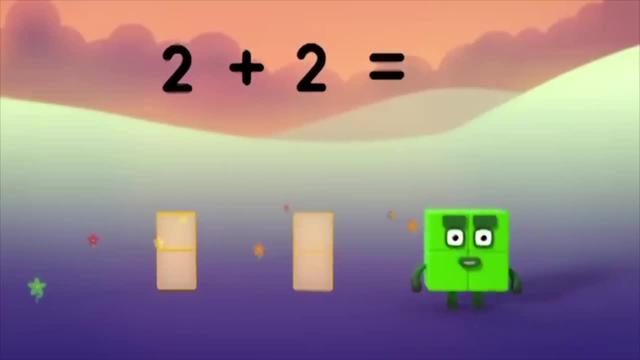 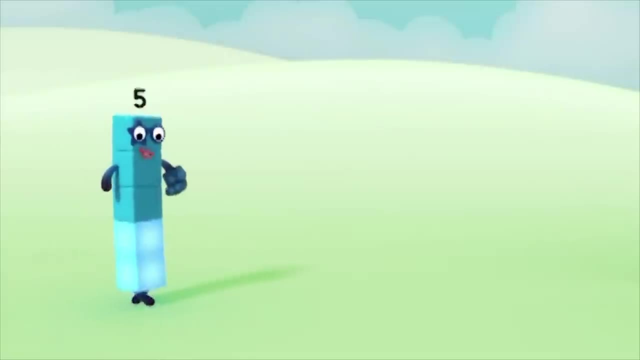 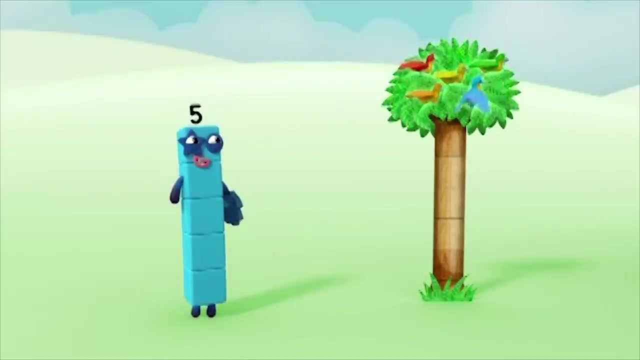 And the whole of me is four, And the whole of me is four. I'm a square. look. Four sides, four corners, One, two, three, four, five. Here I am and I am five: One, two, three, four, five. 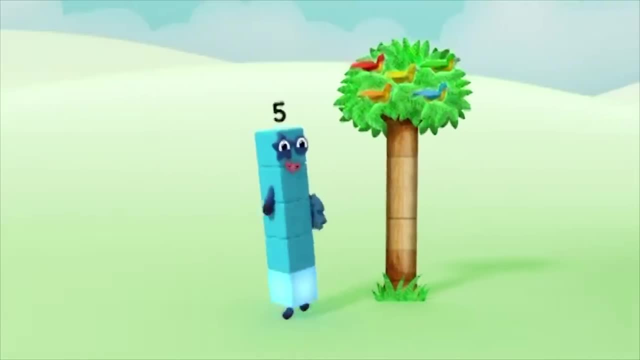 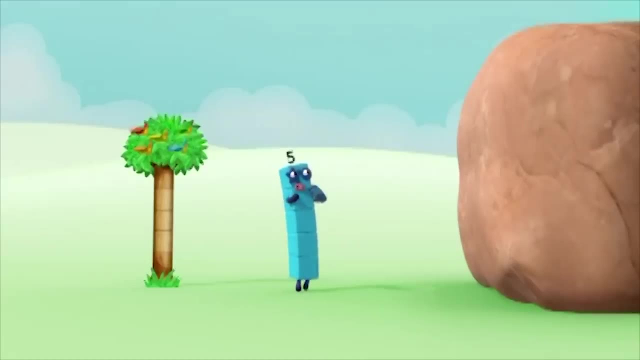 Five little birds have just arrived. One, two, three, four, five. What a wonderful day to be alive. A giant rock in front of me. How can I get where I need to be? What is that silly sucking sound? Oh, look a hole so big and wide. 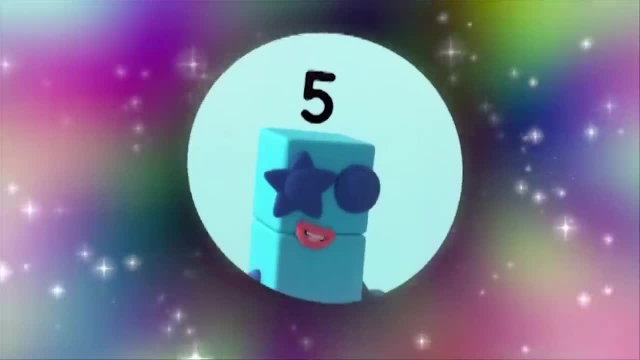 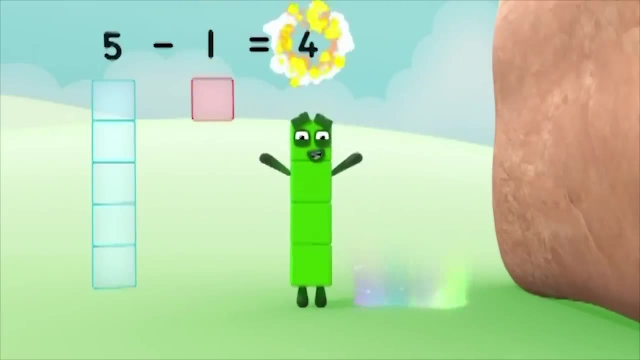 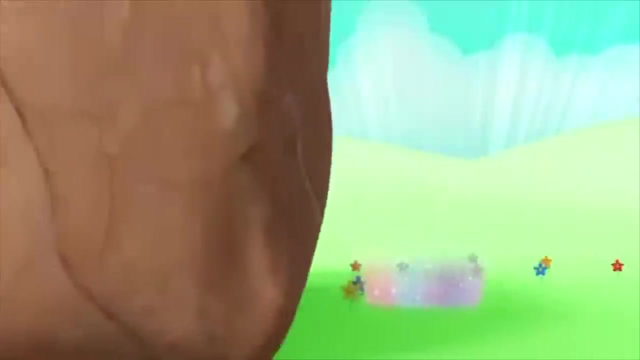 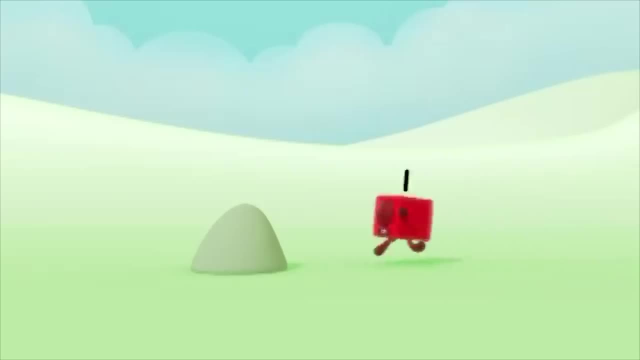 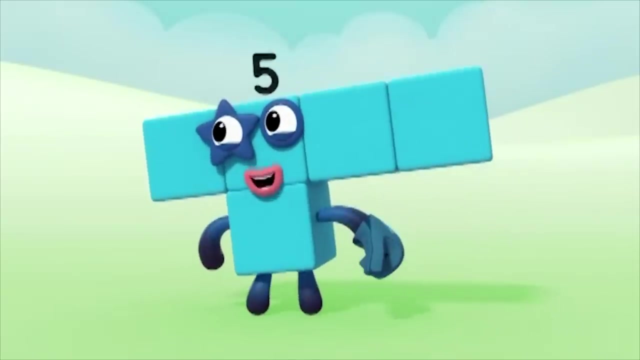 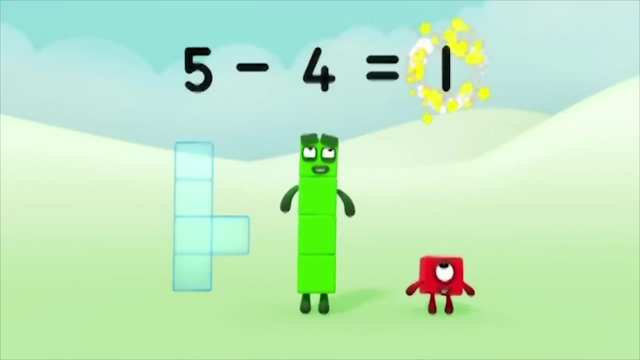 Rock. Ha Ha, Rock, Rock Ha. Oh, Whoa, One Plus four Equals Five. Found you Amazing. Can you find me again? Five Minus four Equals one, Come on, Rock. 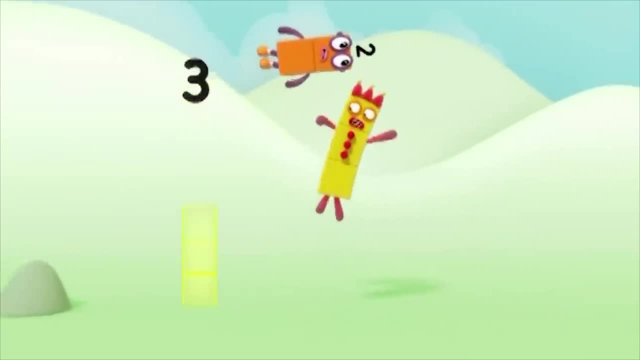 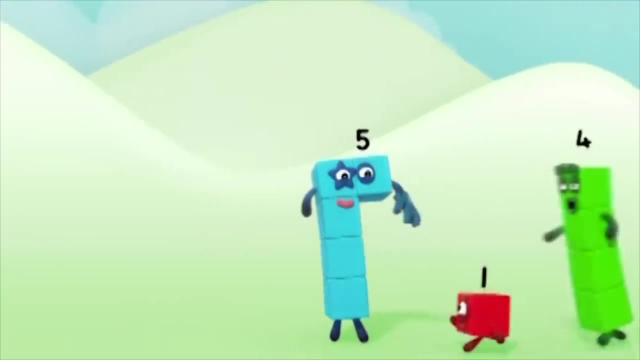 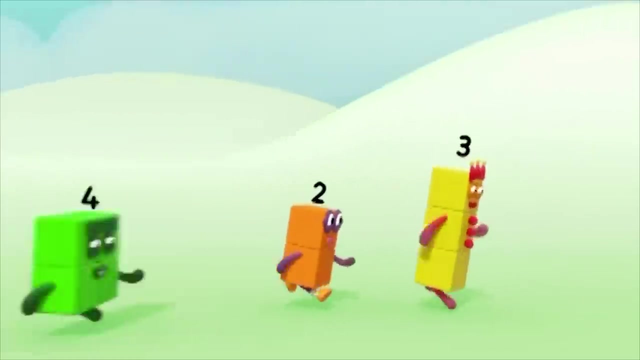 Ooh, Ah, Ooh. Three Plus two Equals Five. Aaaaaaah, Found you Fantastic. Can you find me again? Ooh Aaaaah. Five Minus two Equals three, Aaaaaaah. 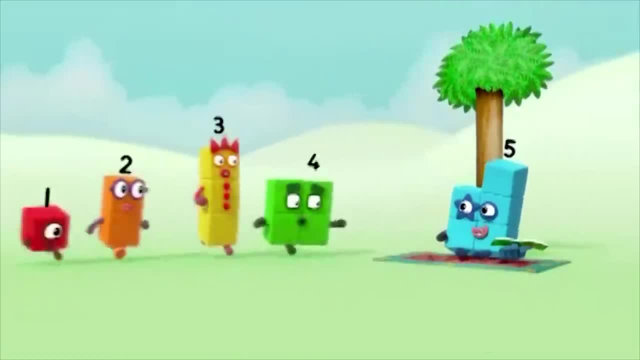 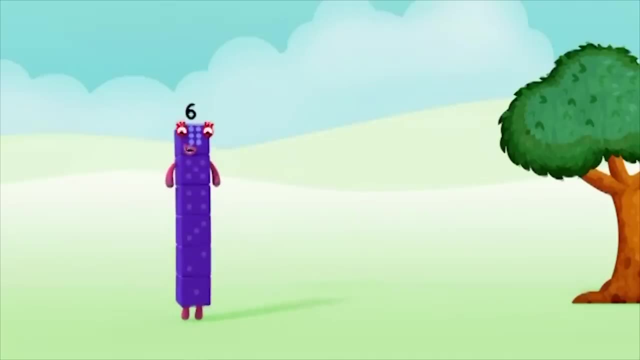 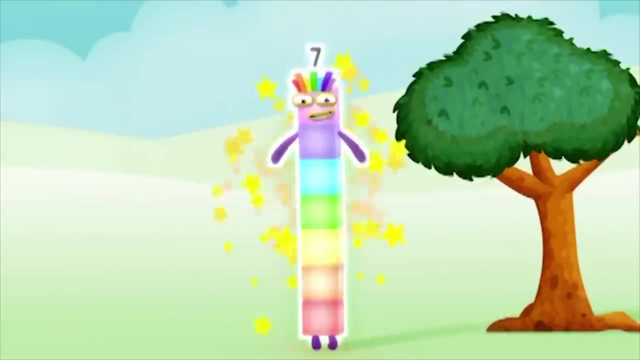 Argh, Aaaaaaah, Found you. Aaaaaah, Ha, Ha, Ha. Now let's add another one. Six Plus one equals seven. I am seven and I'm playing in the sun. making rainbows Is my idea a fun? 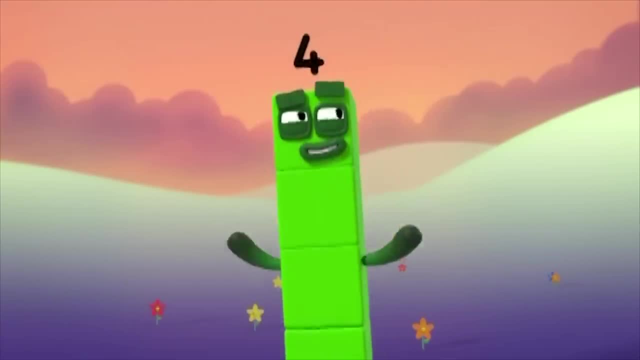 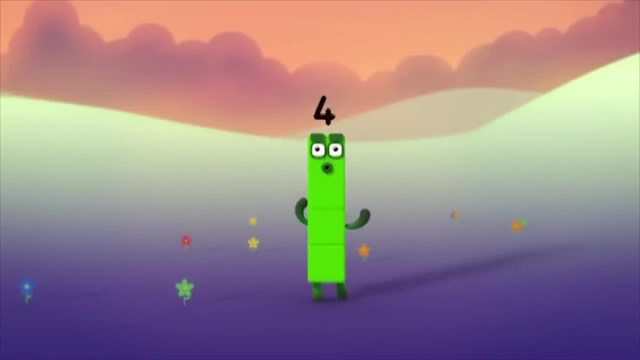 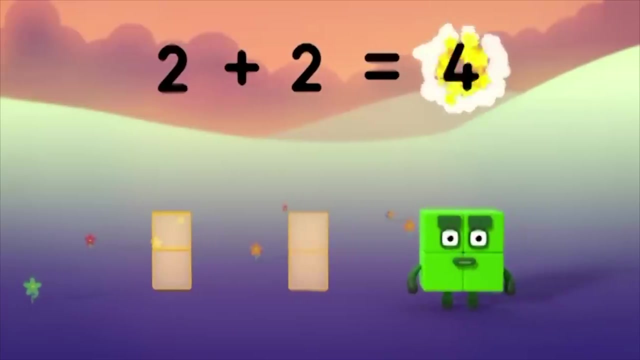 Now here is something more That's different from before. Two is a part of me And two is a part of me, And the whole of me is four. Watch, I'm two And I'm a part. I'm two And I'm a part, And the whole of me is four. 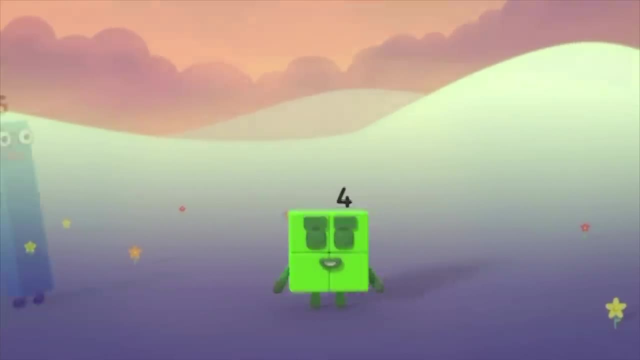 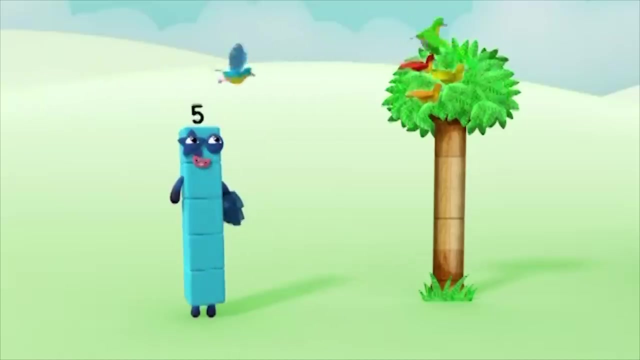 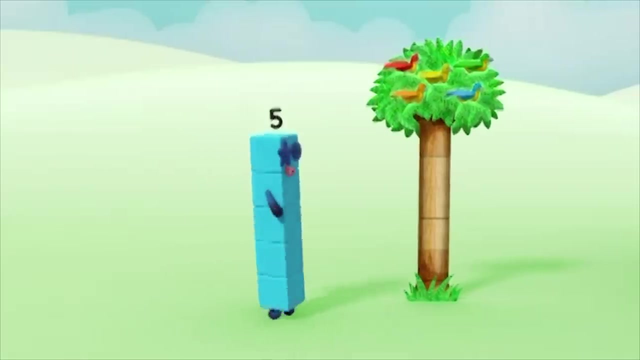 I'm a square. look, Four sides, Four corners. One, two, three, four, five. Here I am, I am five. One, two, three, four, five. Five little birds have just arrived. One, two, three, four, five. What a wonderful day to be alive. 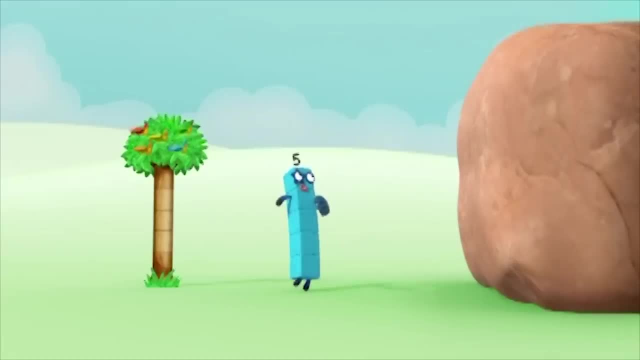 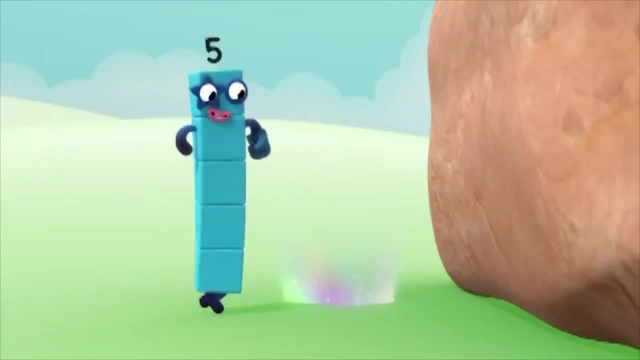 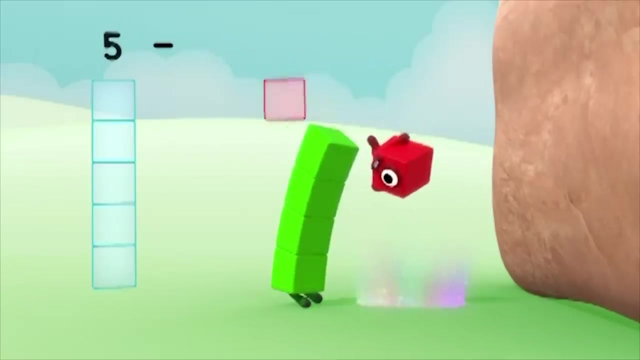 A giant rock in front of me. How can I get where I need to be? What is that silly sucking sound? Oh, look a hole So big and round. Why is it there? I do not know. I wonder what is down below Five minus one. 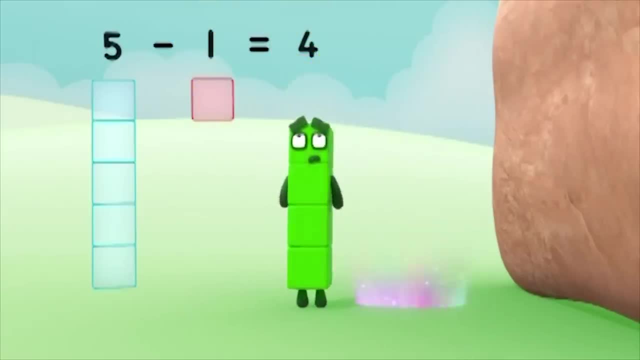 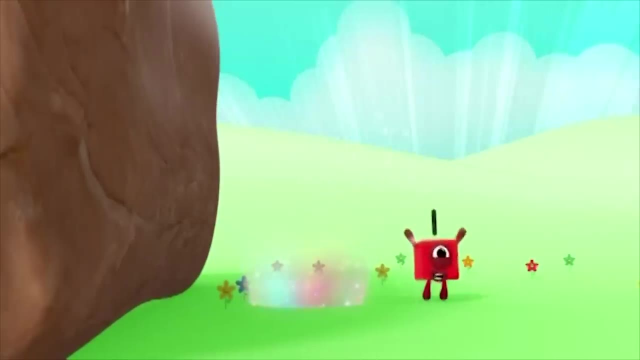 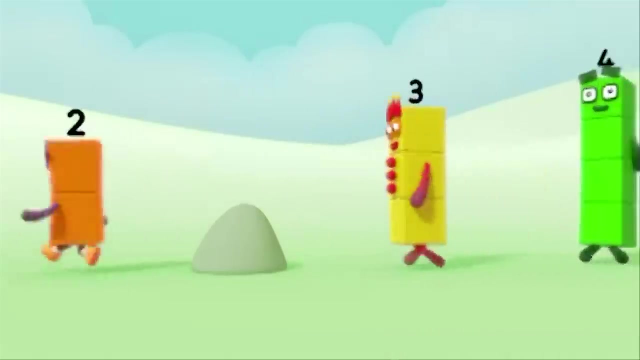 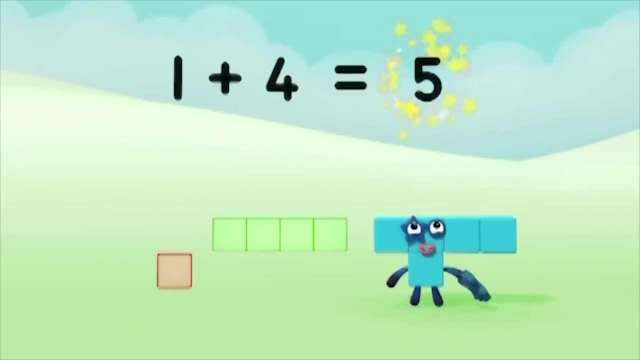 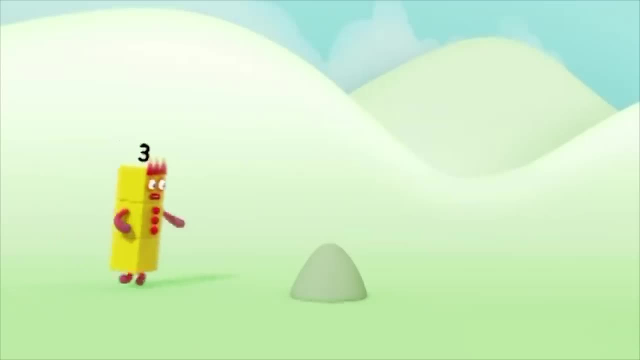 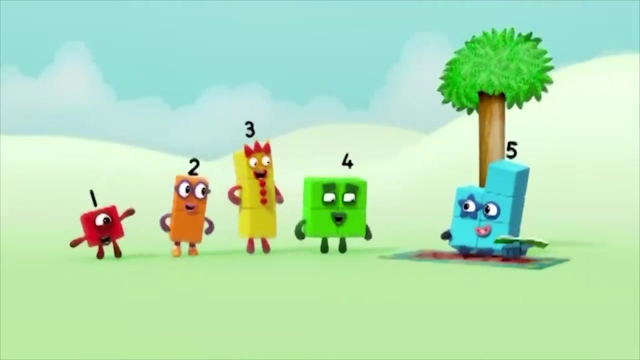 Rock. Three Plus two Equals Four, Five, Five. Found you. Fantastic, Can you find me again? Five minus two Equals three. Five Minus two Equals three. Found you. Now let's add another one: Six Five, One, Two, One, Two, Three, Four, Five, Five, Four, Five, Five, Six Five. 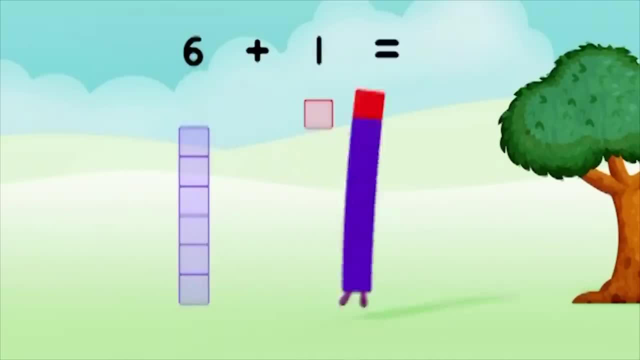 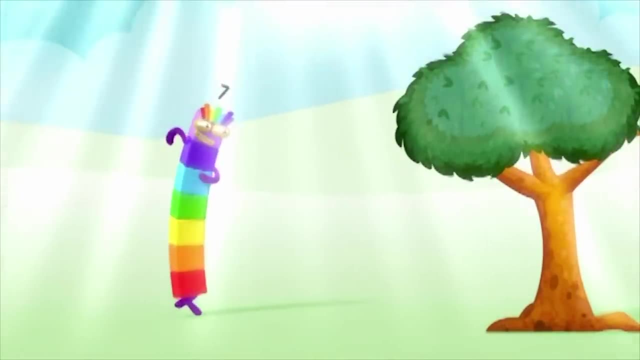 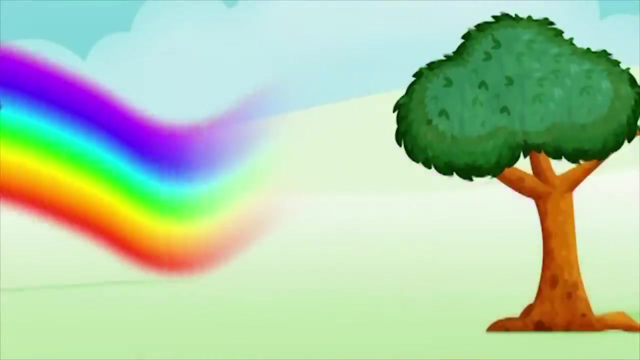 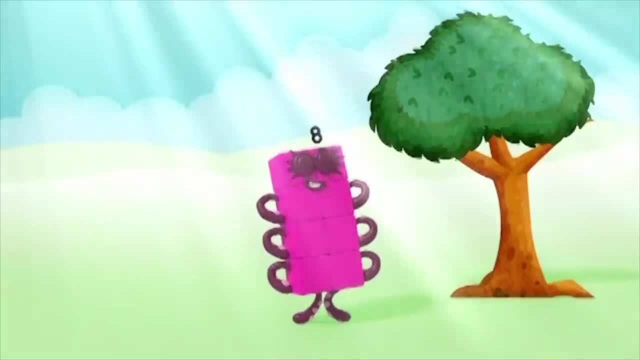 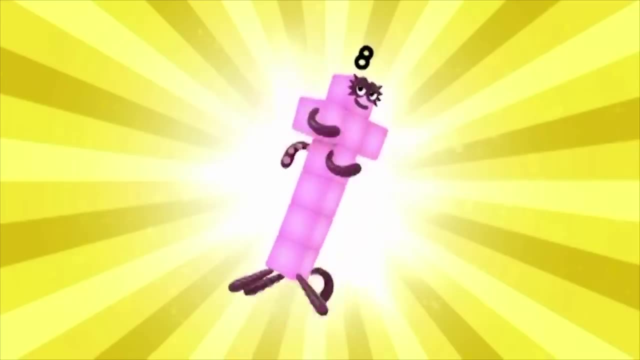 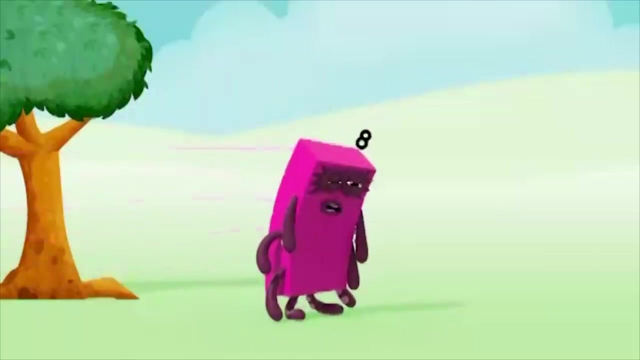 Seven colors. Now let's add another one. Seven Plus one Equals eight. I am eight And I'm playing in the sun being Octoblock. Octoblock: run One, two, three, four, five, six, seven, eight run. Now let's add another one. 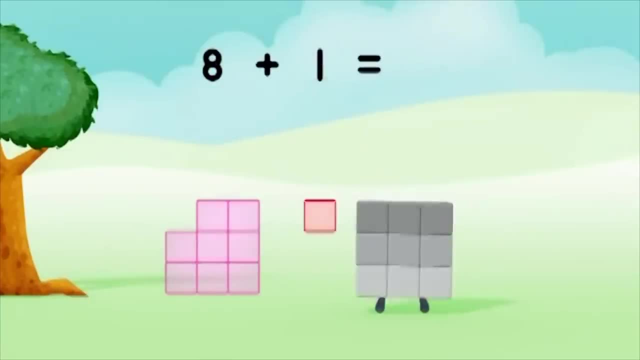 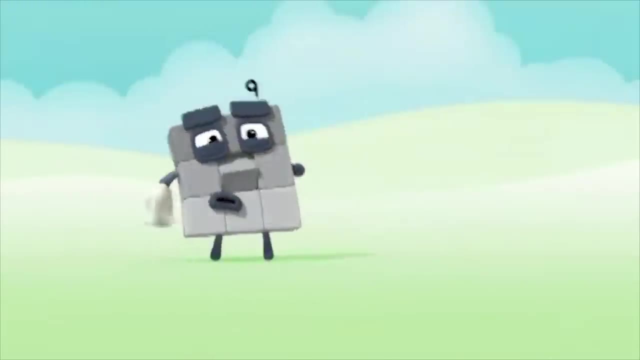 Eight Plus one Equals Nine. I am nine. I am nine And I'm playing in the sun. not sneezing Is my idea of fun. 1, 2, 3, 4, 5, 6, 7,, 8, 9.. 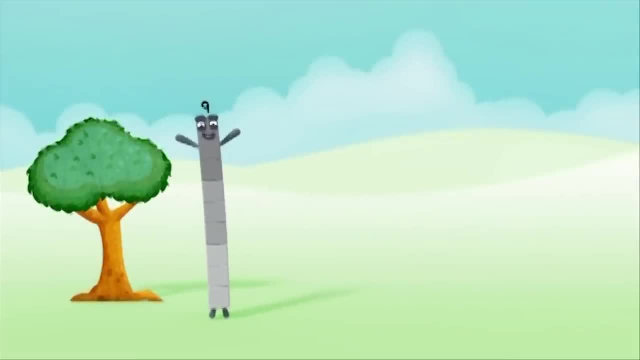 Nine hankies. Now let's add another one. 9 plus 1 equals 10.. I am 10 and I'm playing in the sun. Being 10 is my idea of fun. 1, 2, 3, 4, 5, 6, 7,, 8,, 9,, 10.. 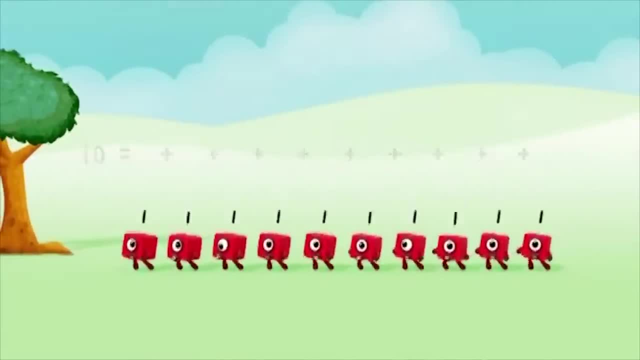 Ten blocks, We're ten ones and we're playing in the sun. Making friends is our idea of fun. 1, 2, 3, 4, 5, 6, 7,, 8,, 9,, 10.. 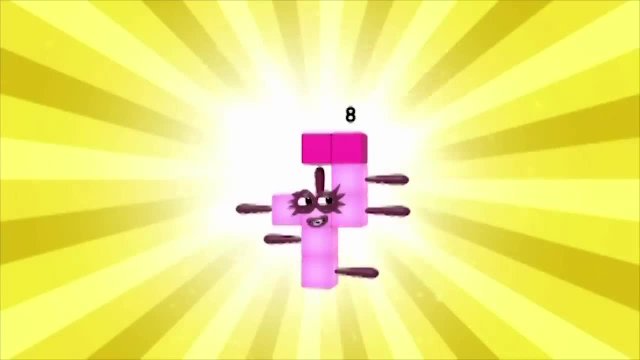 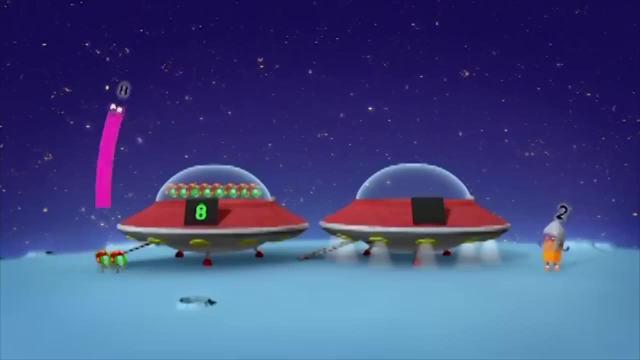 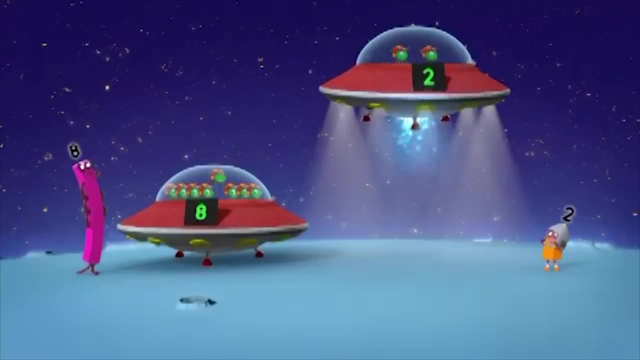 Octoblock: build 1,, 2,, 3,, 4,, 5,, 6,, 7,, 8.. Build Two flying saucers. Good work, Oh, come back, it's not starting, Whoa. 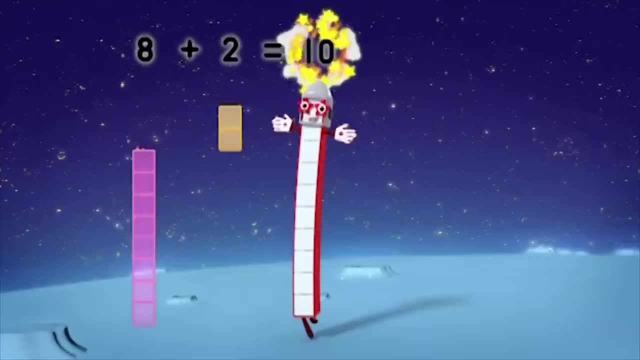 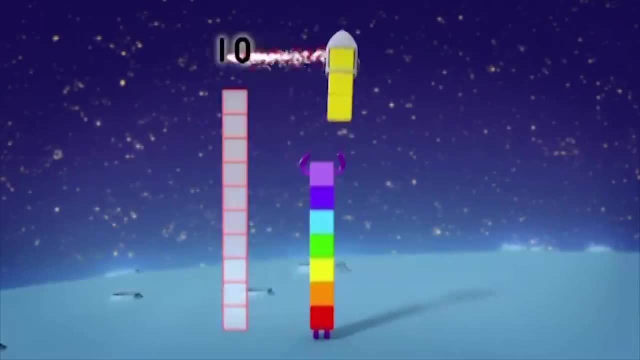 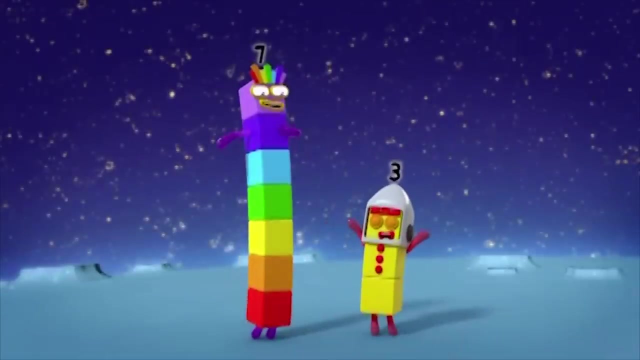 8 plus 2 equals 10!. Here I am, number 10.. Time to make some friends again. 10 equals 7 plus 3.. We're on the moon. seven and three. We're so lucky. look at me. 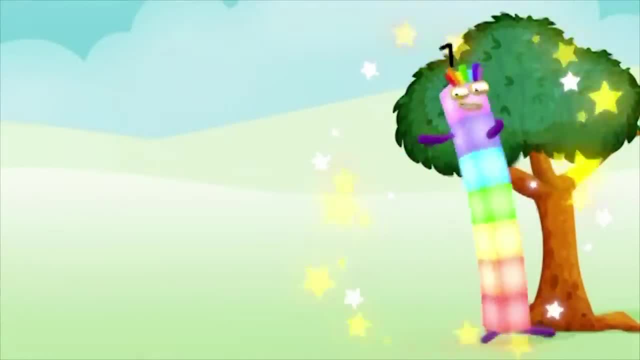 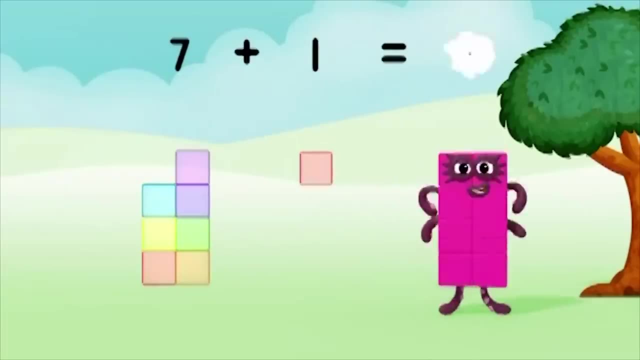 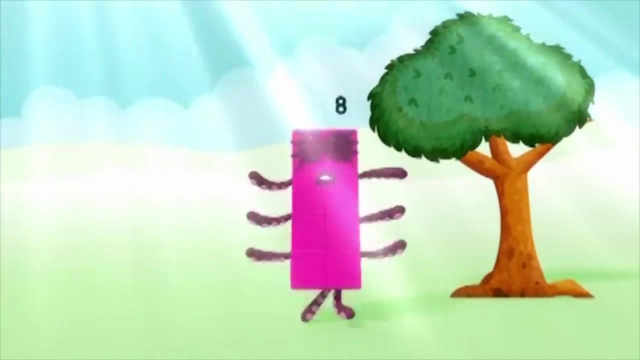 One, two, three, four, five, six, seven, Seven colours. Now let's add another one. Seven plus one equals eight. I am eight and I'm playing in the sun. being Octoblock Is my idea a fun? 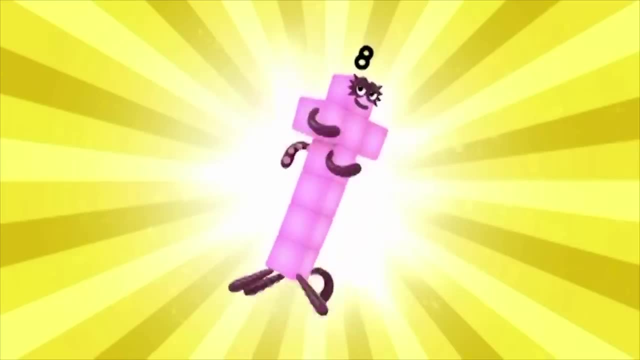 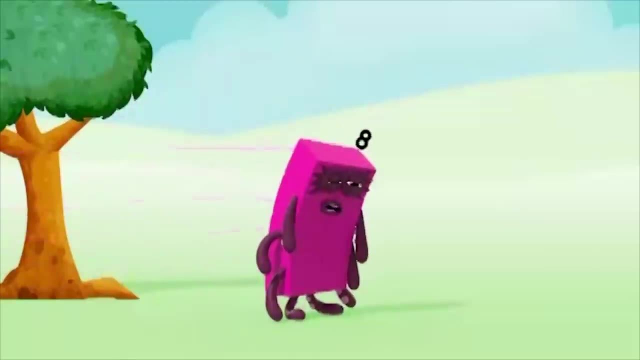 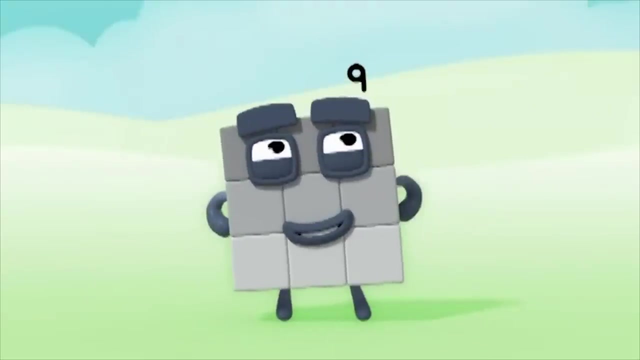 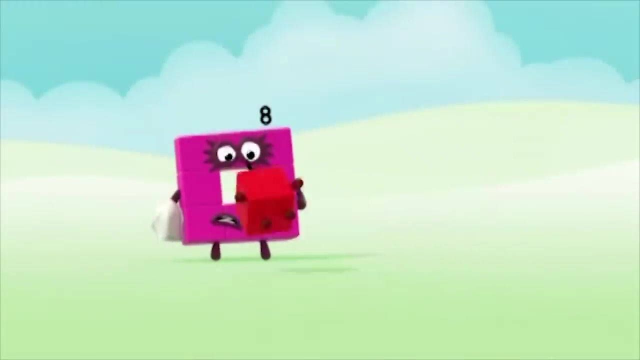 Octoblock run One, two, three, four, five, six, seven, eight run. Now let's add another one. Eight Plus one equals nine. I am nine, I am nine and I'm playing in the sun, not sneezing. 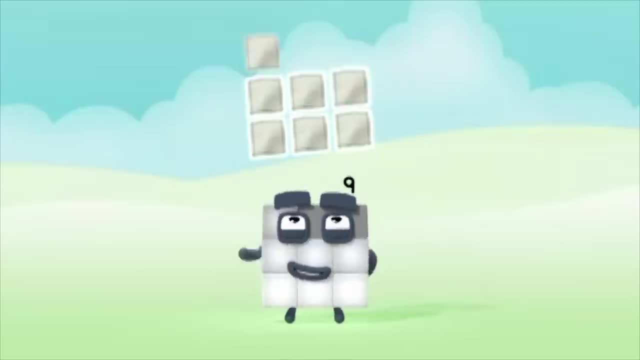 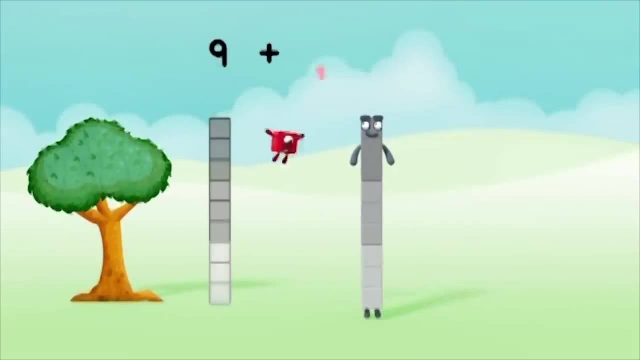 Is my idea a fun: One, two, three, four, five, six, seven, eight, nine, Nine hankies. Now let's add another one. Nine plus one equals ten. I am ten and I'm playing in the sun being ten. 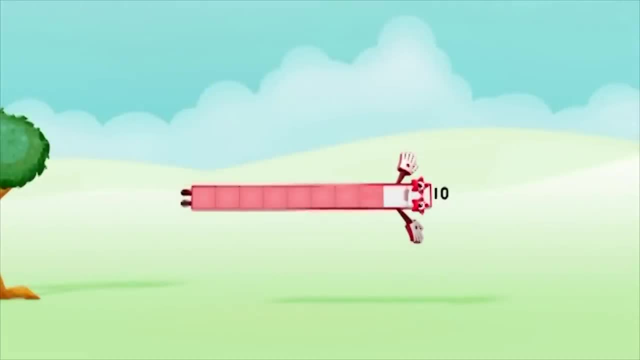 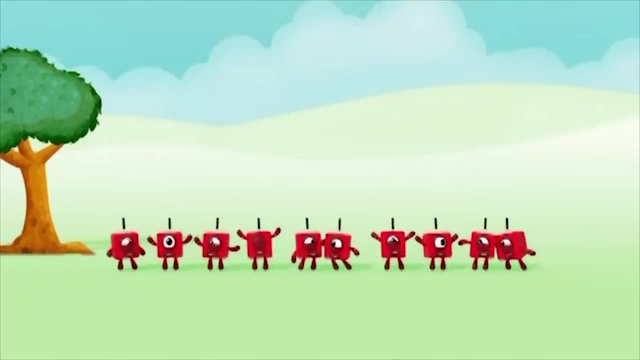 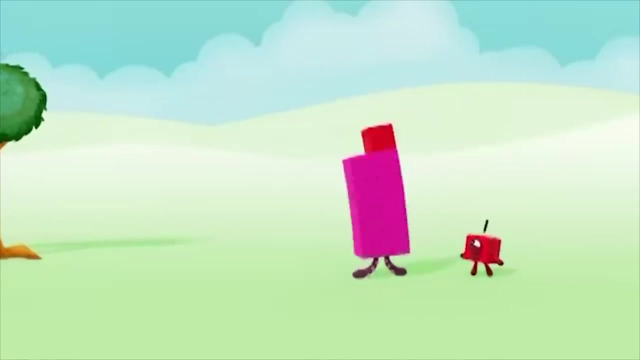 Is my idea a fun. One, two, three, four, five, six, seven, eight, nine, ten, Ten blocks. We're ten ones and we're playing in the sun. Making friends is our idea of fun. One, two, three, four, five, six, seven, eight, nine, ten. 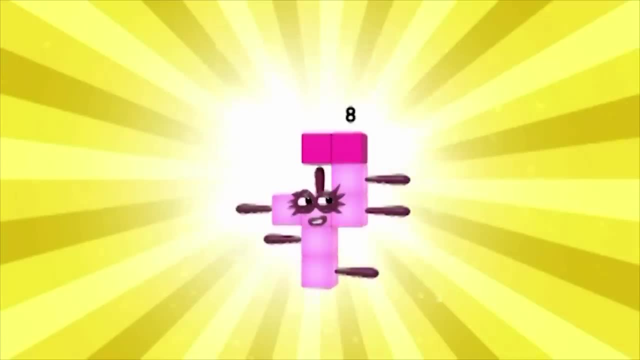 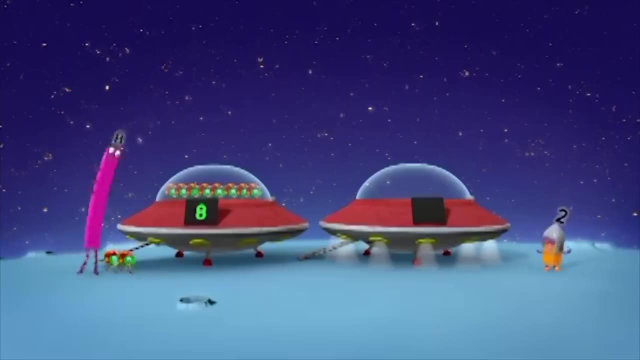 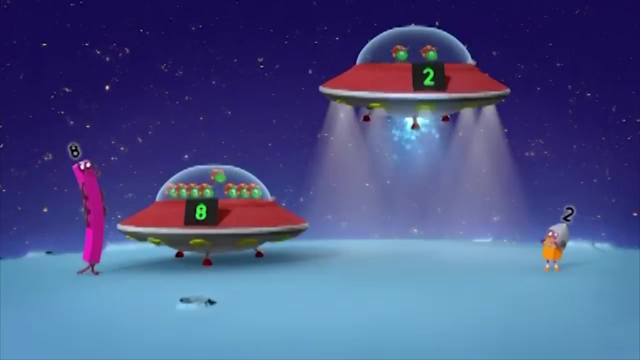 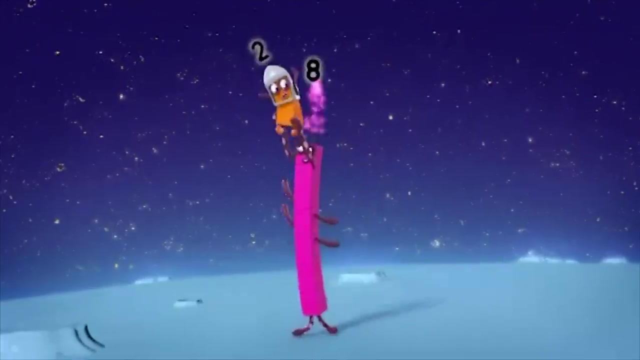 Octoblock: build One, two, three, four, five, six, seven, eight, Build, Build Two flying saucers. Good work, I'll come back. It's not starting. Eight plus two equals Ten. 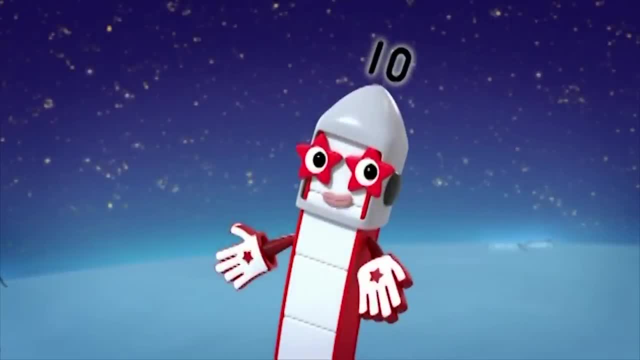 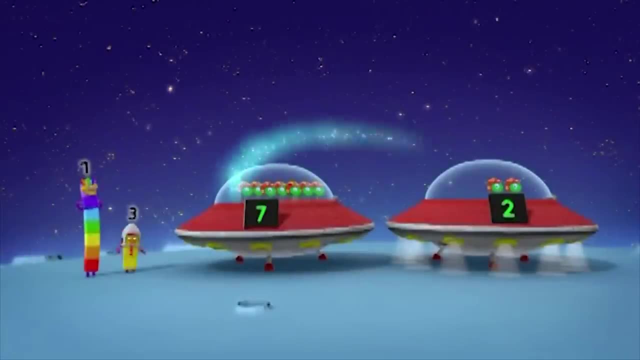 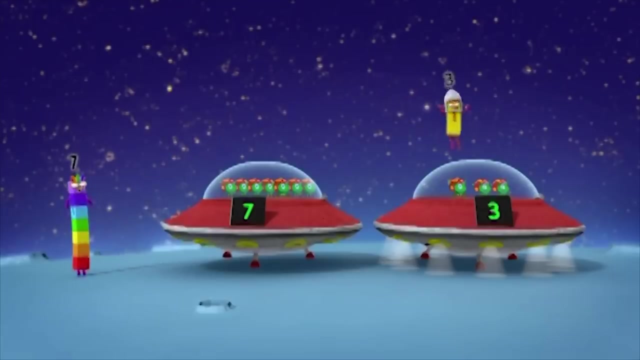 Here I am, number ten: Time to make some friends again. Ten equals seven plus three- We're on the moon. Seven and three, We're so lucky. Look at me. Look at that. There's the on button. That was lucky. 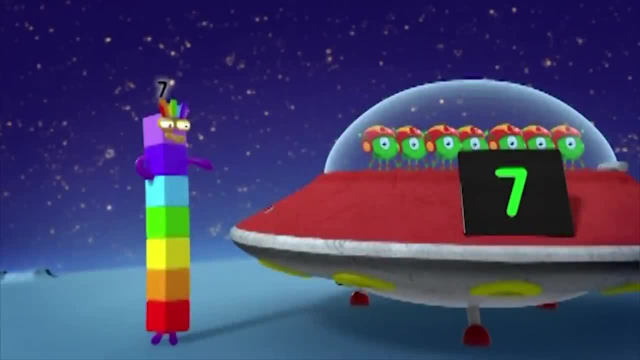 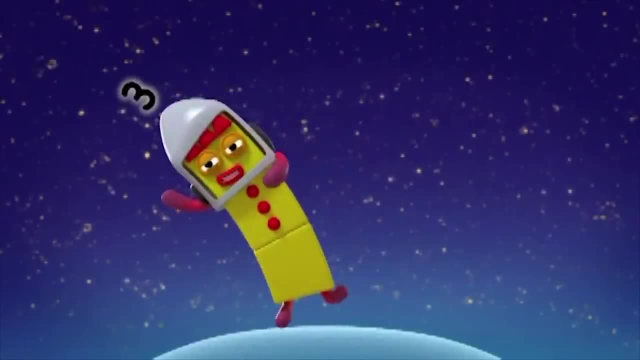 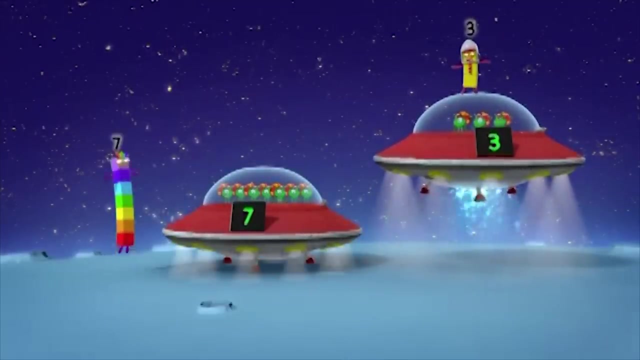 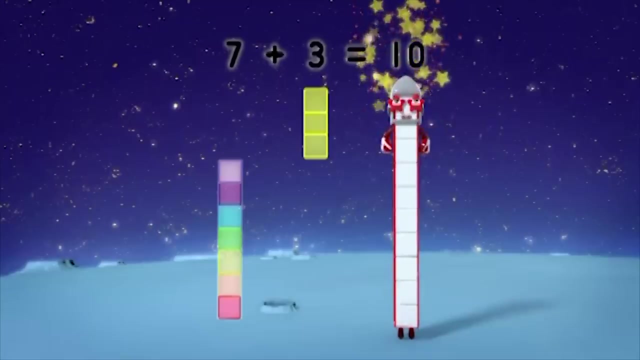 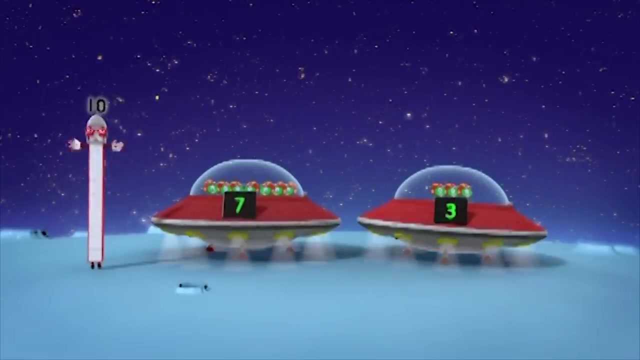 Woo-hoo, Look at that. There's the on button. That was lucky, Ready, steady, Blast off. Oh, it's too heavy. 7 plus 3 equals 10!. It's 10 again. Wait and see who my next two friends will be. 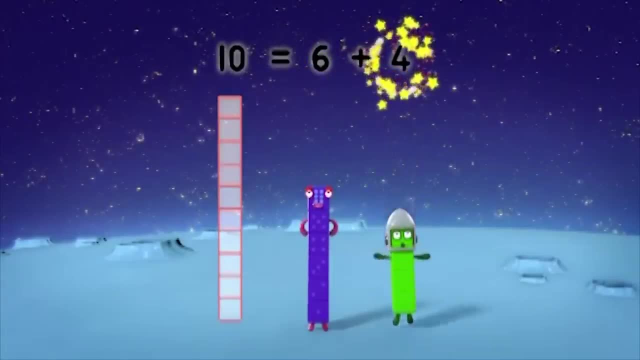 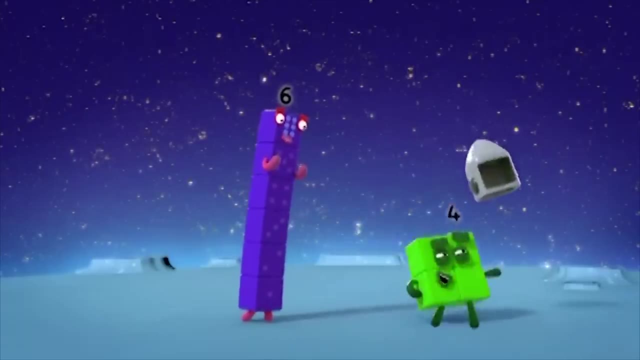 10 equals 6 plus 4.. 10 equals 6 plus 4.. 10 equals 6 plus 4.. We're on the moon. six and four. We really couldn't ask for more. Let's play a game. 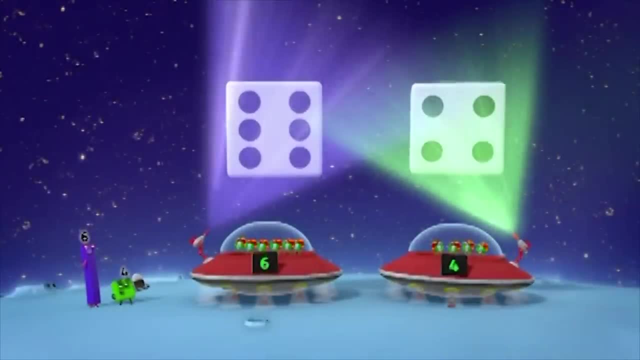 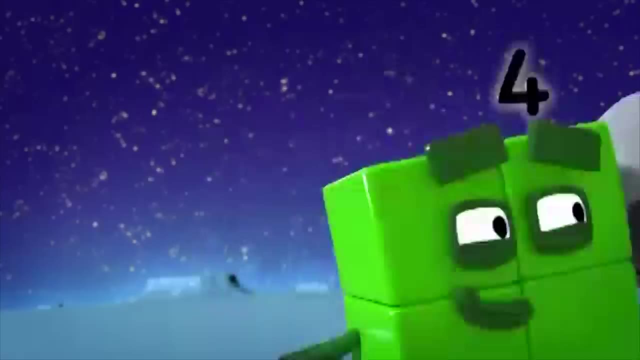 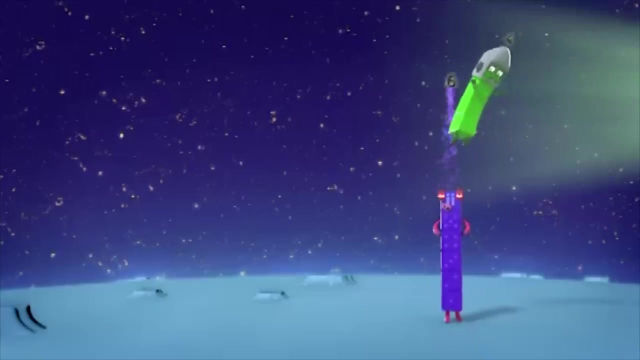 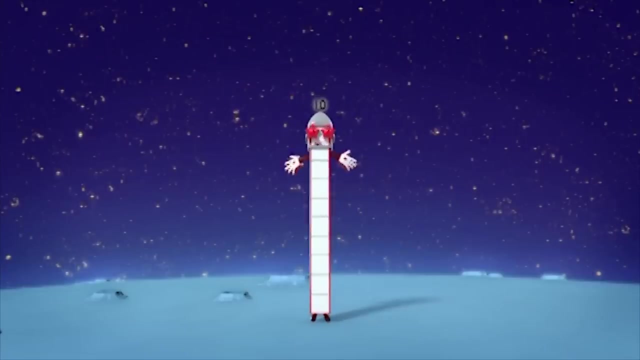 Roll the dice and Whoa, Whoa, That was so cool. Still too heavy, Oh Oh, 6 plus 4 equals 10.. Quick, before our visit ends, We've just got time for two more friends. 10 equals 5 plus 5.. 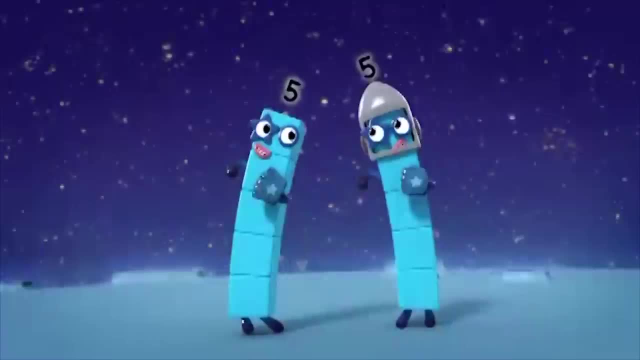 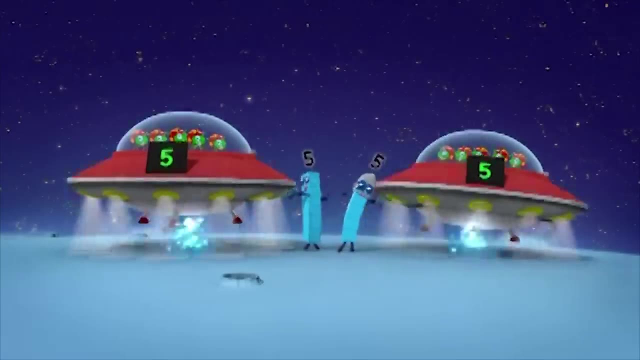 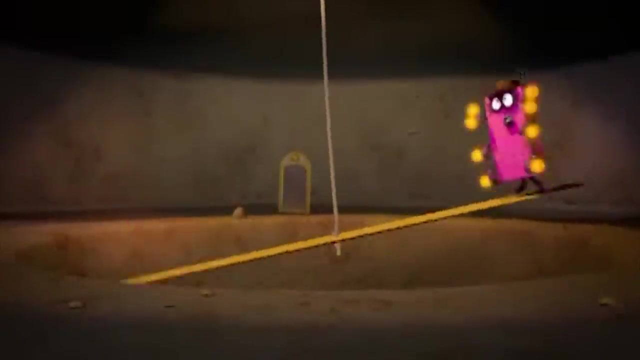 We're on the moon. five and five. It sure feels great to be alive. Let's give them a hand. Woo-hoo, High five, Oh, Woo-hoo-hoo-hoo-hoo-hoo. Octoblock splits in half. 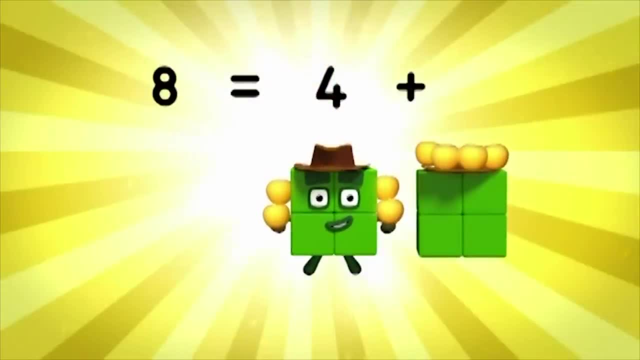 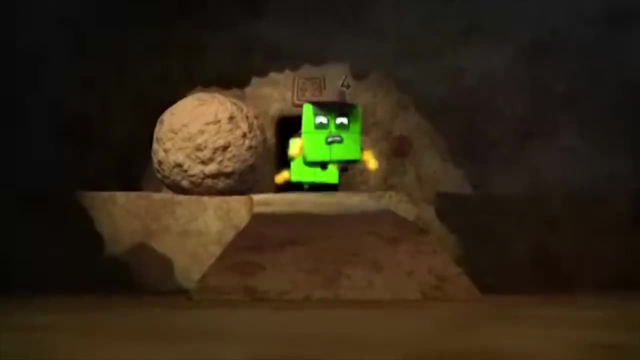 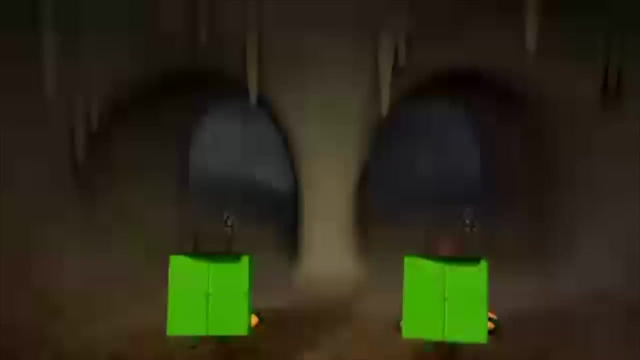 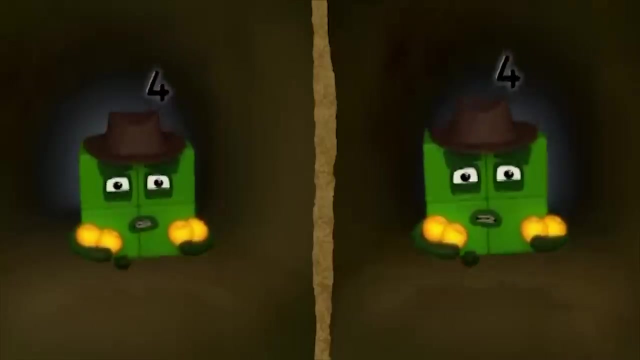 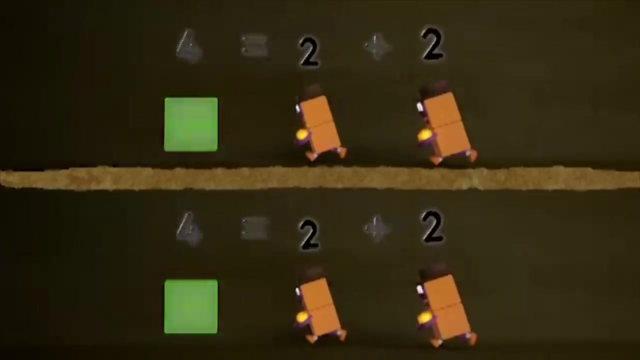 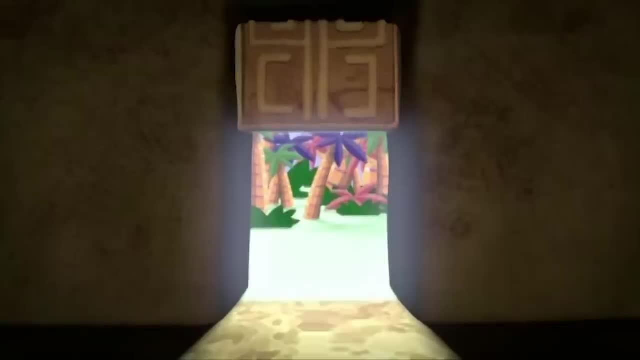 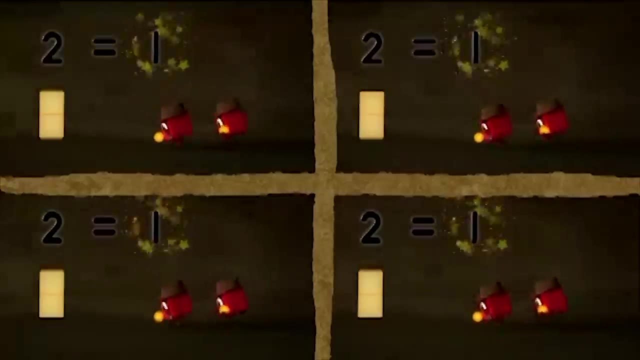 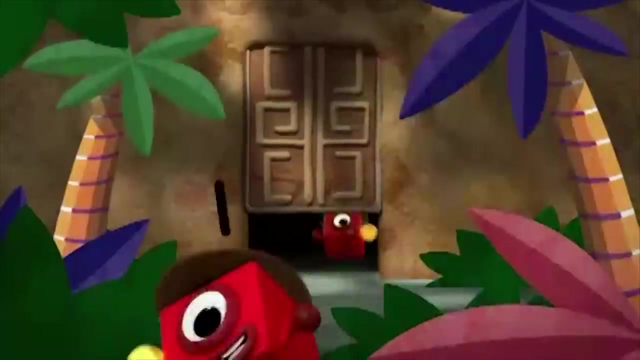 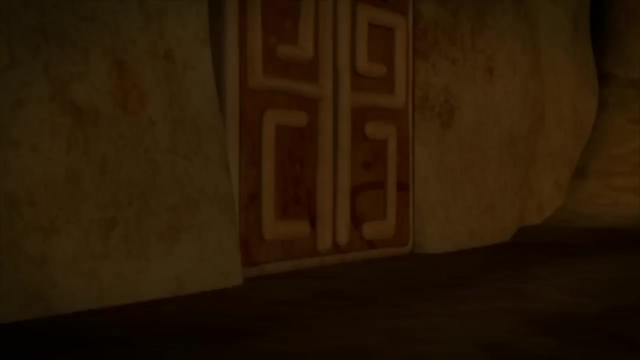 We're not going to make it. What now? Split in half, Two equals 1 plus 1.. Woo-hoo, Ha-ha. Five, Five, Five, Five, Shhhh, Shhhh, Ha, Ha, Ha. 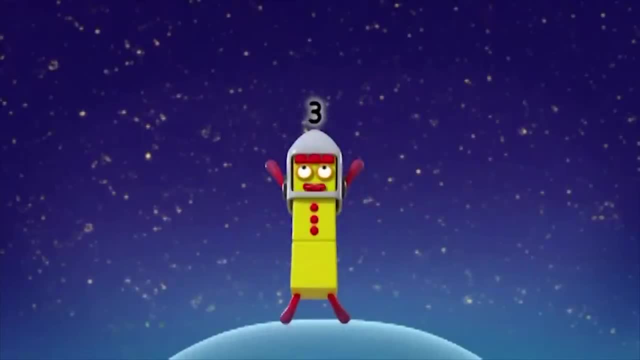 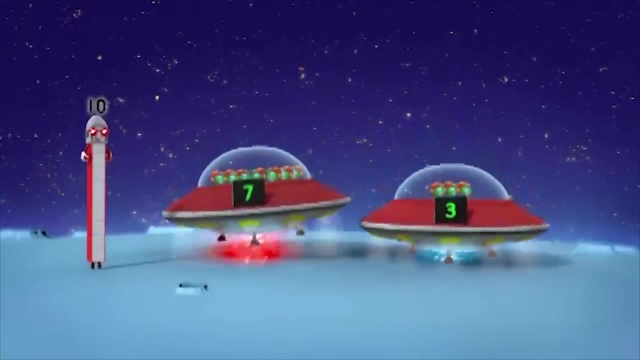 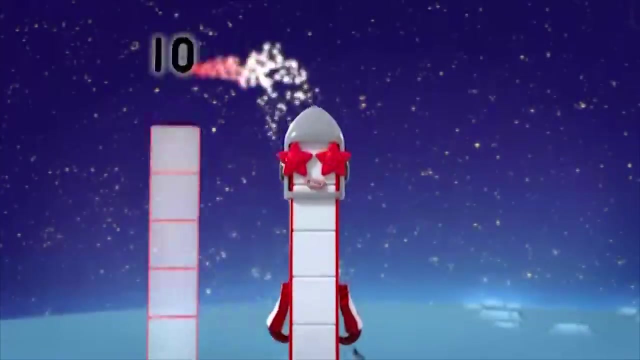 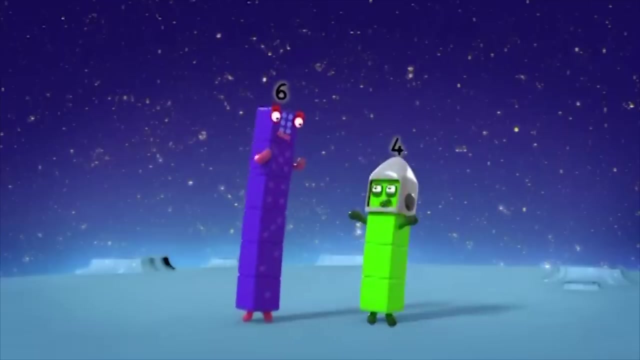 Ready, steady, blast off. It's too heavy. Seven plus three equals ten. It's ten again. Wait and see who my next two friends will be. Ten equals six plus four. We're on the moon. Six and four. We really couldn't ask for more. 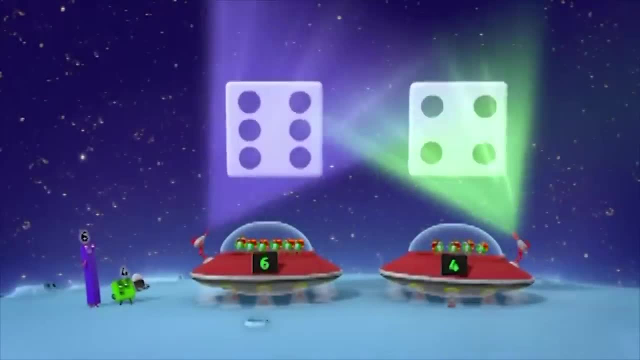 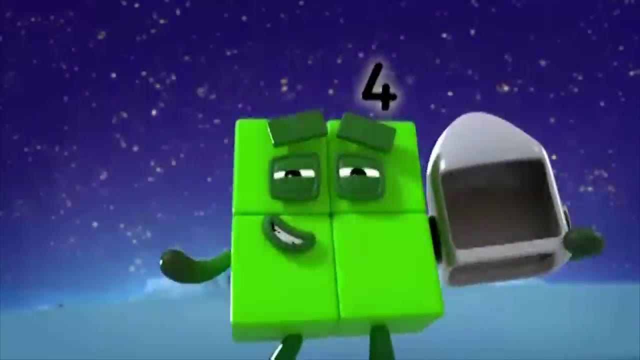 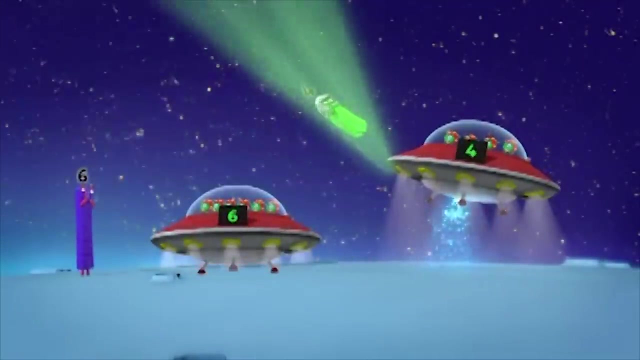 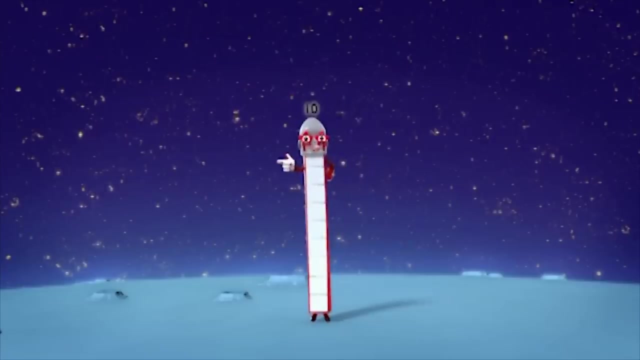 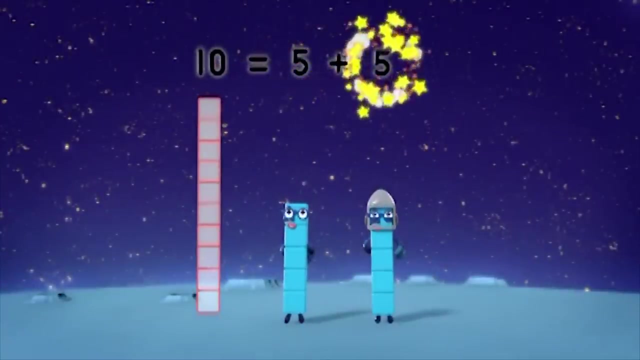 Let's play a game: Roll the dice. and That was so cool. Still too heavy. Six plus four equals ten. Quick, before our visit ends, We've just got time for two more friends. Ten equals five plus five. We're on the moon. 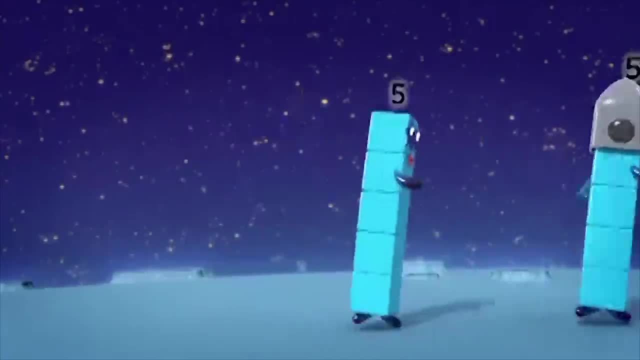 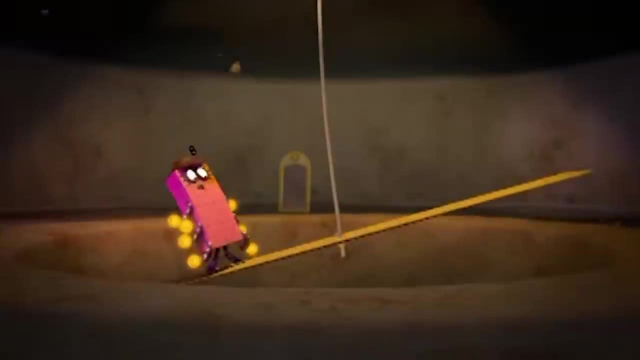 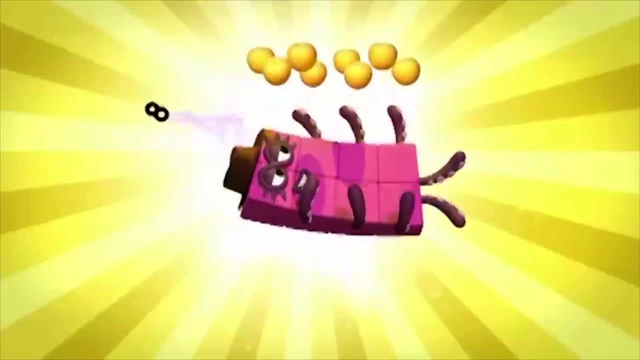 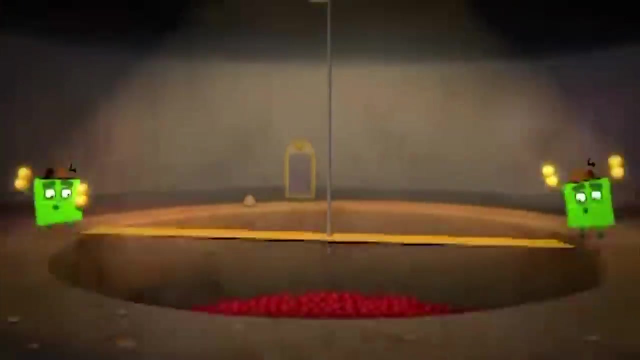 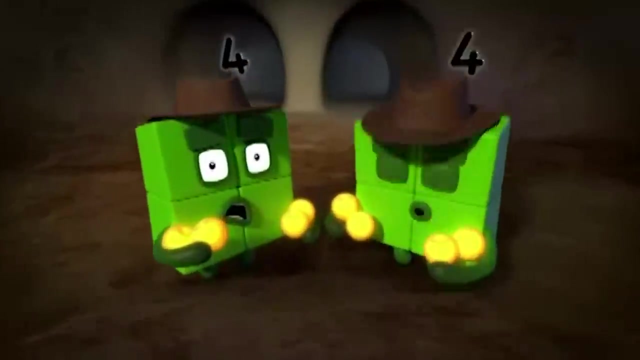 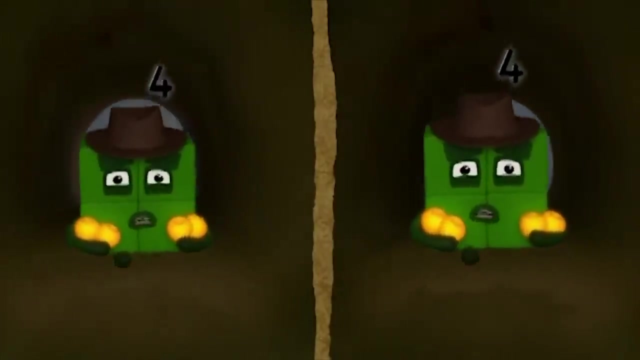 Five and five. It sure feels great to be alive. Let's give them a hand. Ah, High five. Octoblock splits in half. Eight equals four plus four. Giant rounding alert. Ah, Look out, The river sneaks. 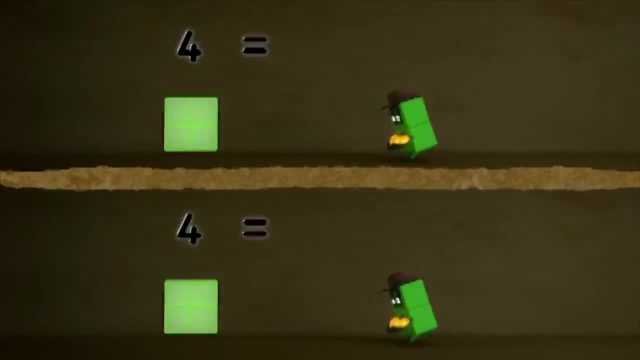 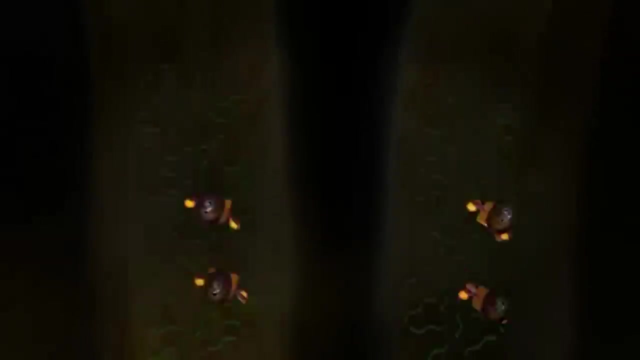 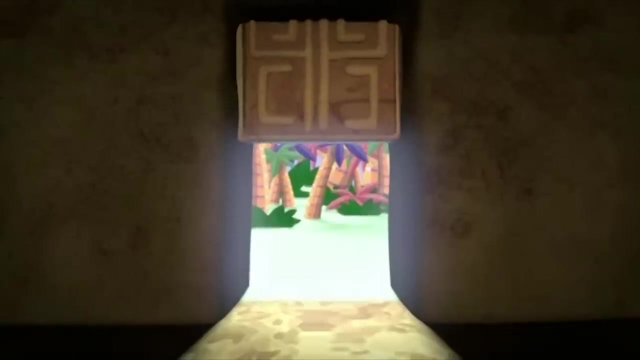 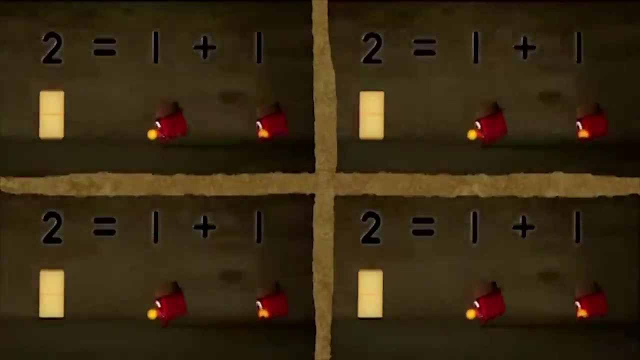 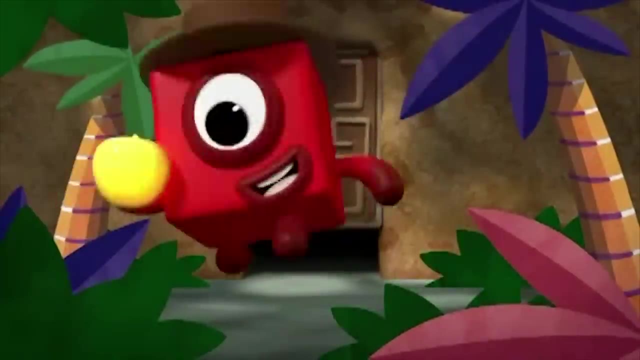 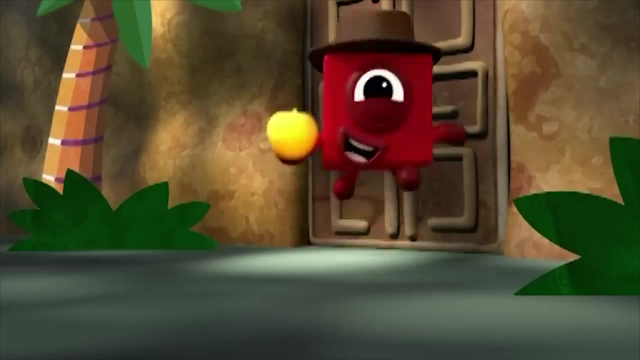 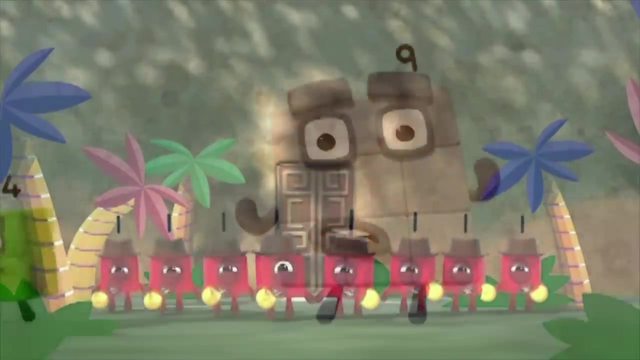 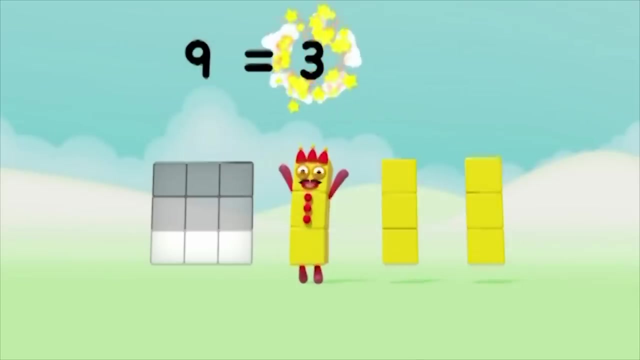 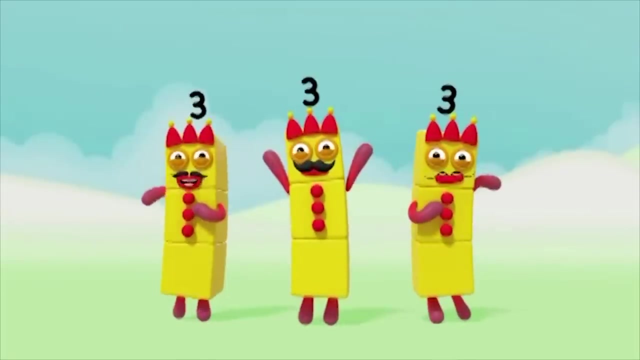 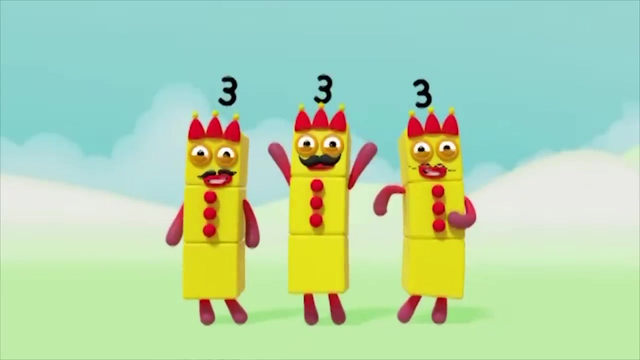 One plus one, What? Five, Five, Five, Five, Pawn Phew Nine equals three plus three plus three. Roll up, roll up, roll up. We three are the Three Threes The most amazing, the most incredible, The most extraordinary acrobats in Numberland. 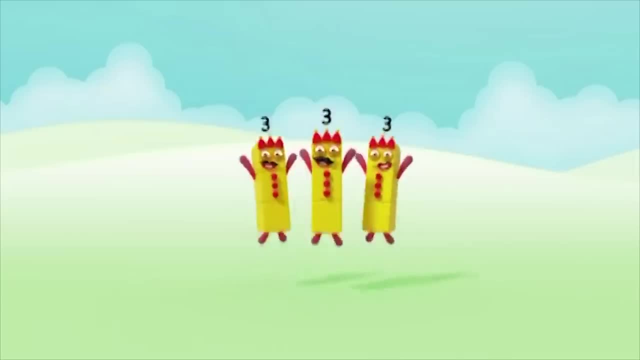 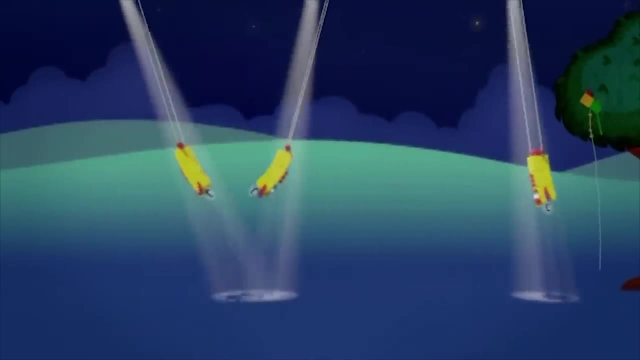 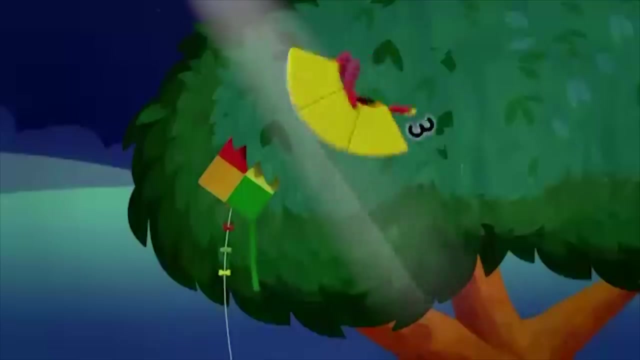 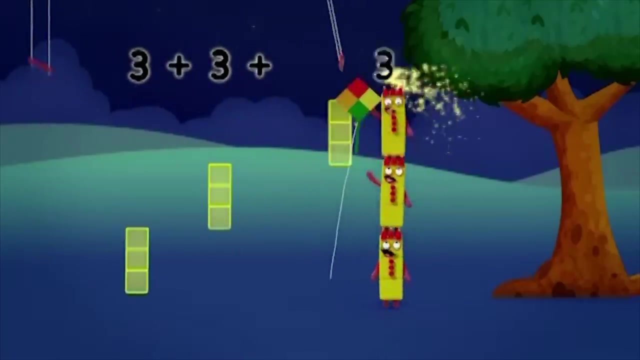 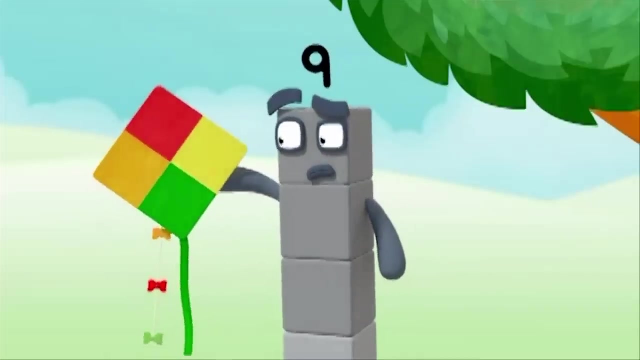 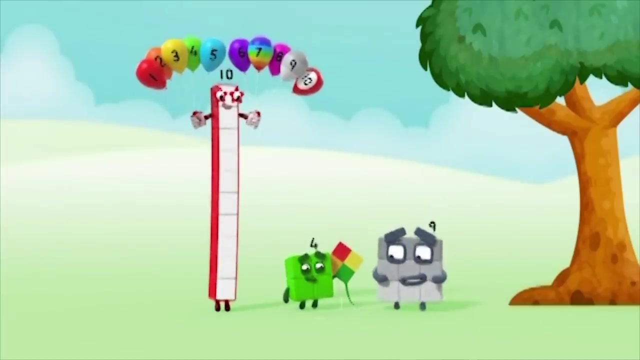 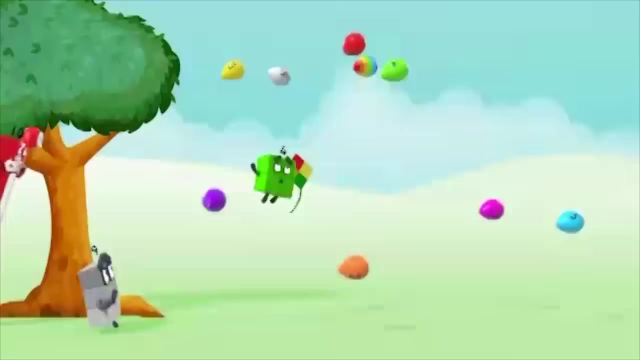 Drumroll please, As we present the Three Threes On the Flying Trapeze: Three plus three plus three equals Nine. Nine, you did it. Did what? Oh yes, It was nothing really Quick. stop them. There are too many, We need help, Help. 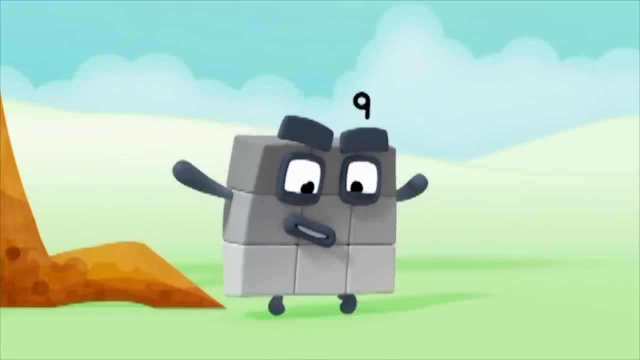 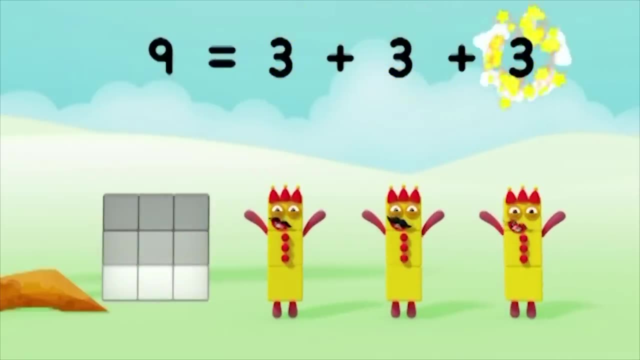 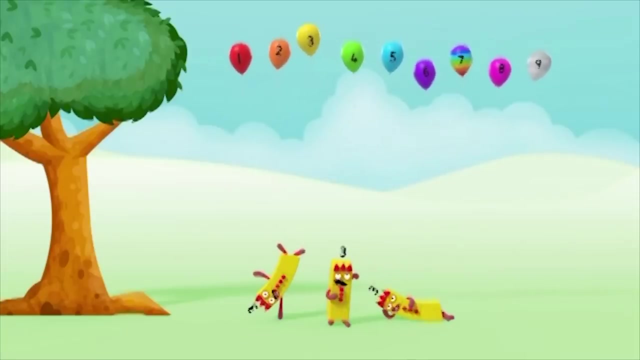 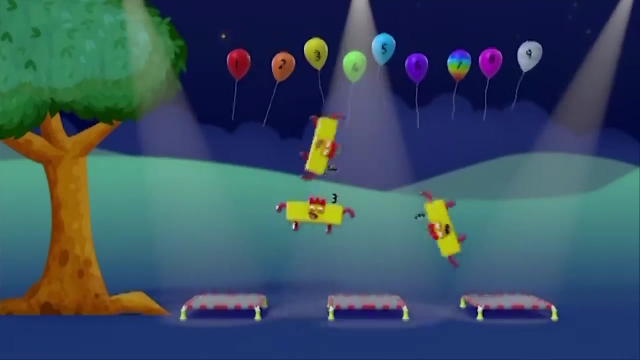 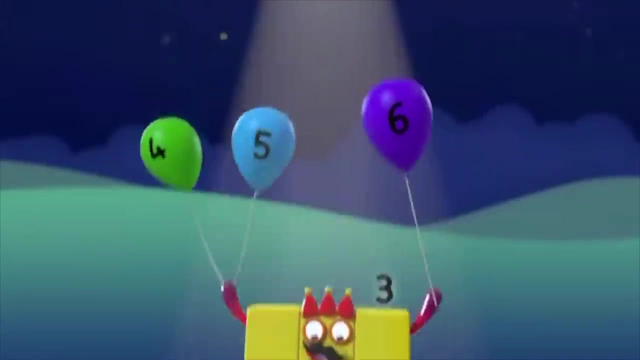 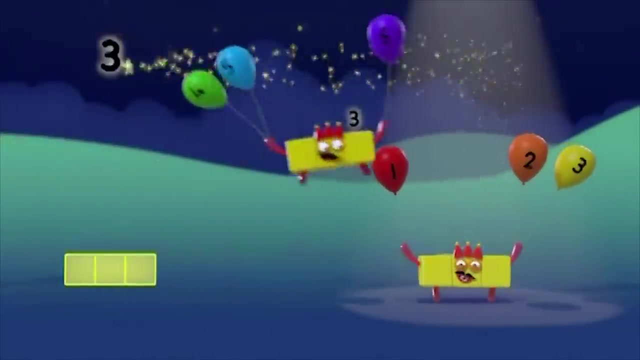 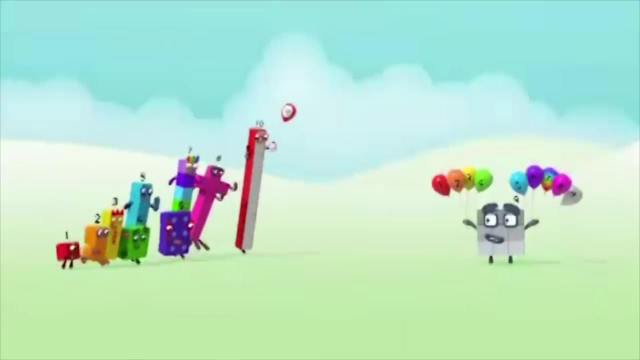 I can do this myself. Nine equals Three plus three plus three. The Three Threes will seize these with great ease. Drumroll please. One, two, three, Four, five, six, seven, eight, nine. Three plus three plus three equals Nine. You did it again. 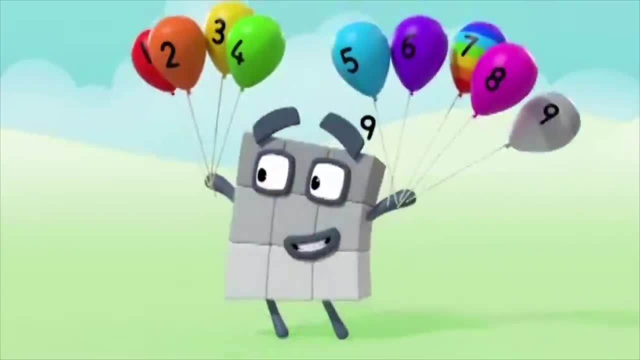 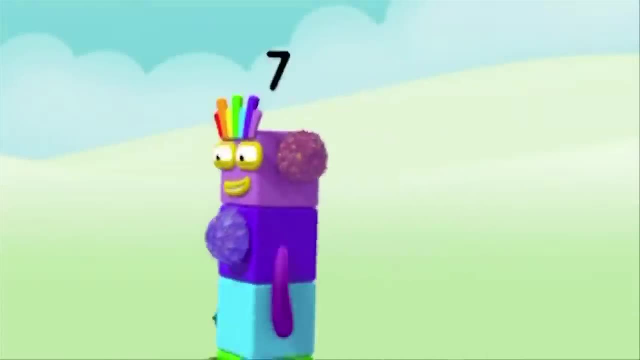 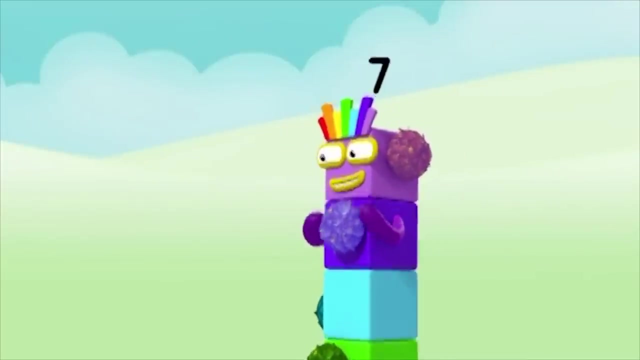 I did, Yes, I did, I did, Yes, I did. Of course I did. Sevens are not ticklish. How lucky is that. Oh, have you all had enough tickling? Why don't you just make sevens then? How? 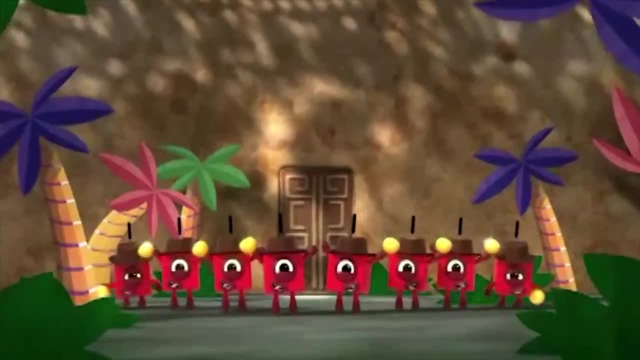 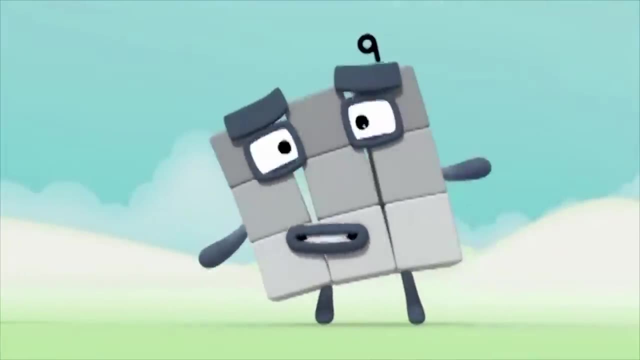 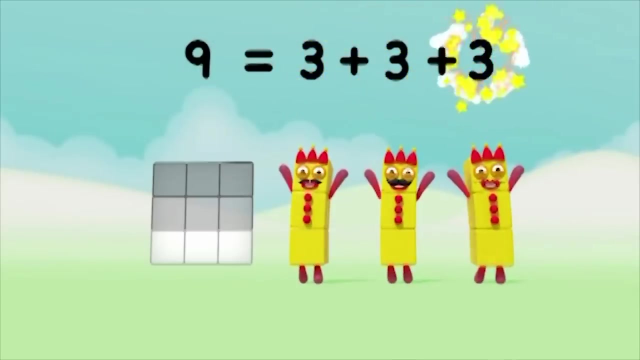 Phew, Ha-ha-ha-ha-ha, Ha-ha-ha-ha, Ha Ha, Ha-ha-ha-ha-ha. Nine equals Three plus three plus three. Woo-hoo, Roll up, roll up, roll up. 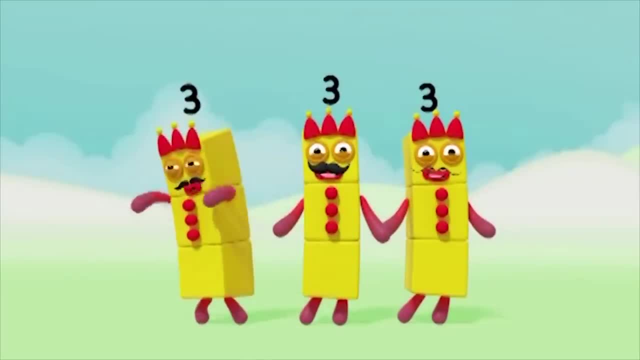 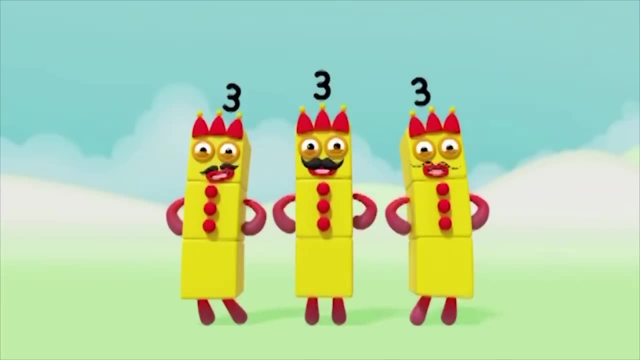 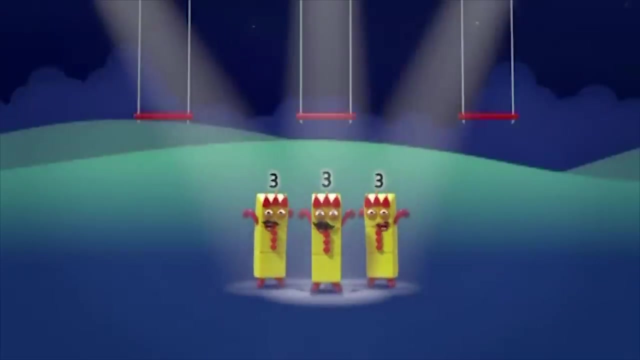 We three are the Three Threes: The most amazing, the most incredible, the most extraordinary acrobats in Numberland. Drum roll please, as we present the Three Threes On the Flying Trapeze: Woo-hoo-hey. 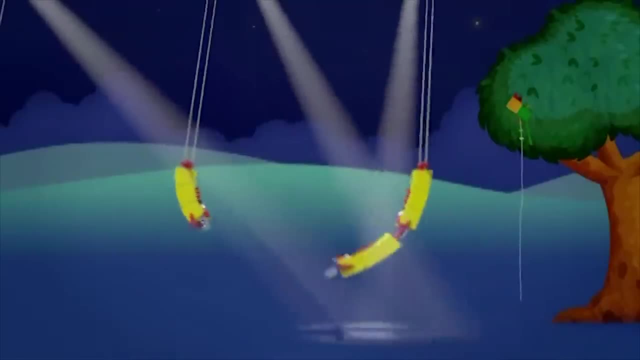 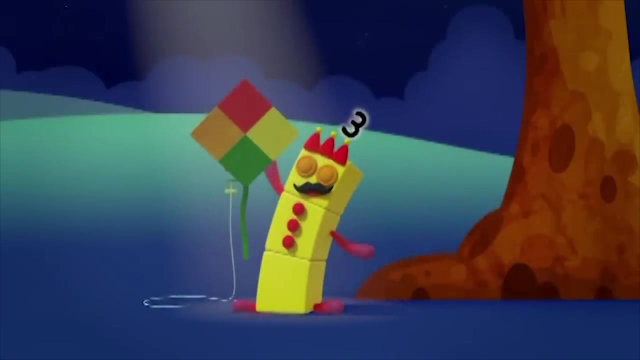 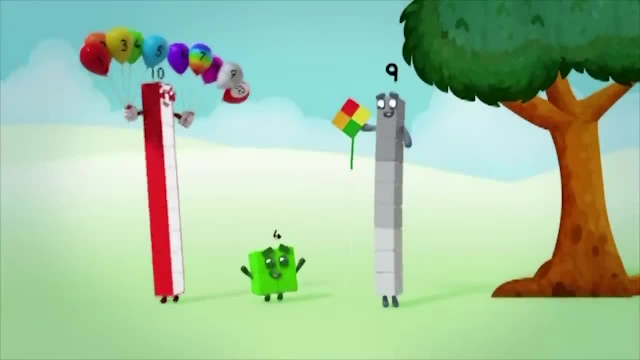 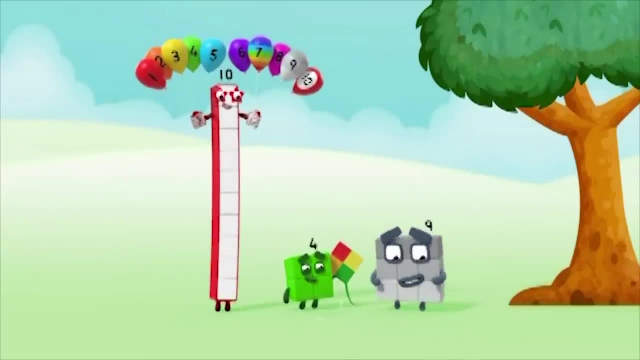 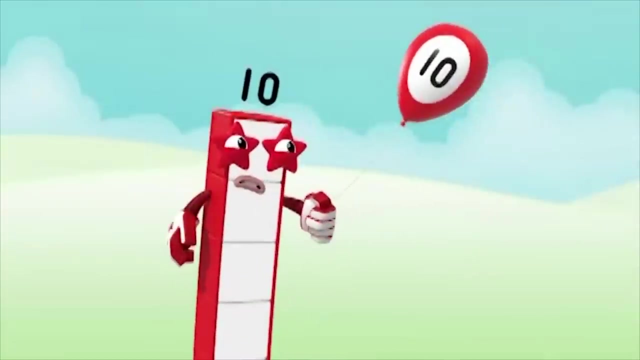 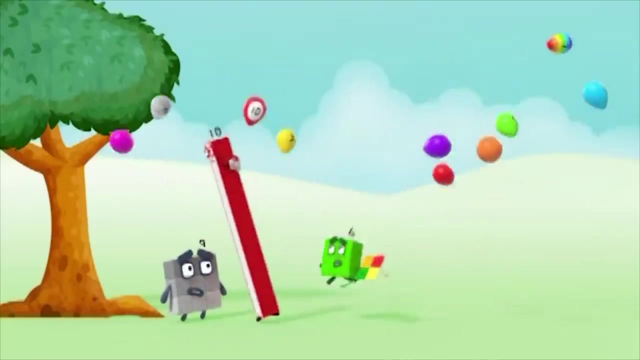 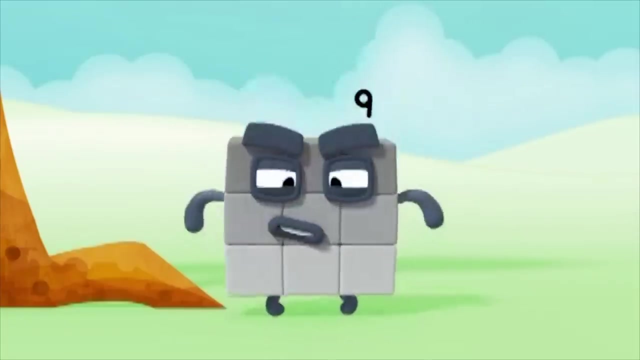 Woo, 3 plus 3 plus 3 equals Nine. Nine, You did it. did what? Oh, Yes, Ha, There are too many. We need help. Help, I can do this myself. Nine equals three plus three plus three. 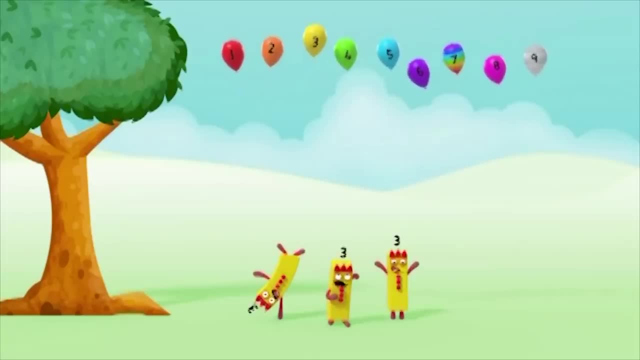 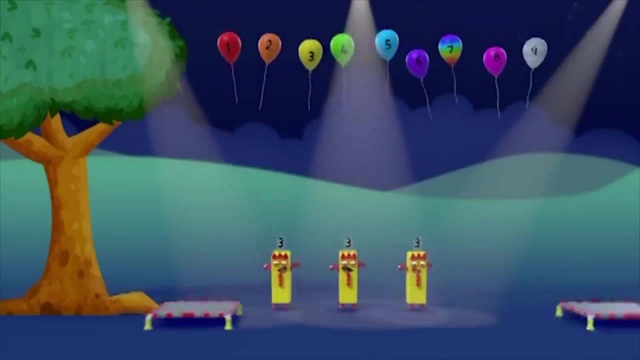 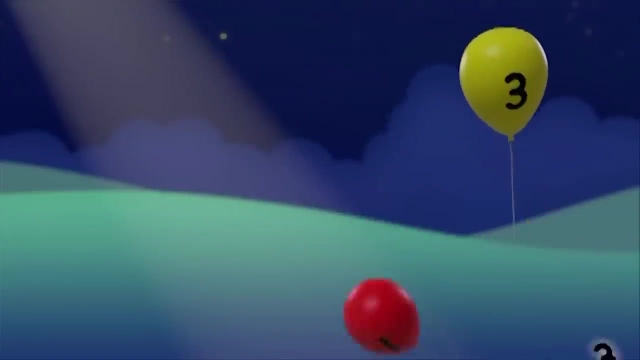 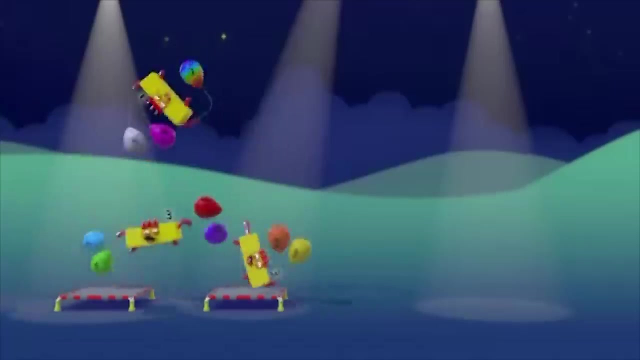 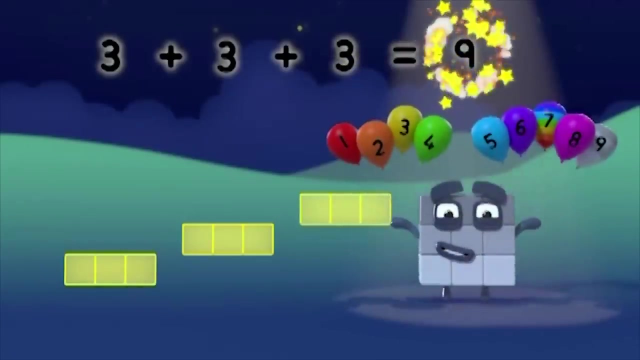 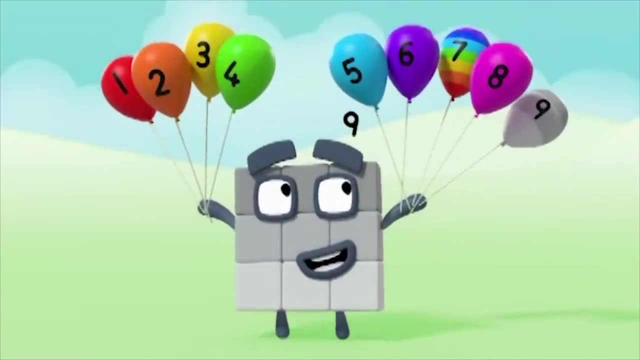 The three threes will seize these with great ease. Drum roll please. One, two, three, four, five, six, seven, eight, nine. Three plus three plus three equals nine. You did it again. I did, Of course. 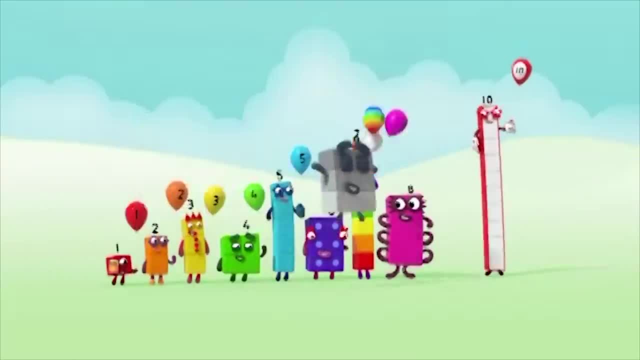 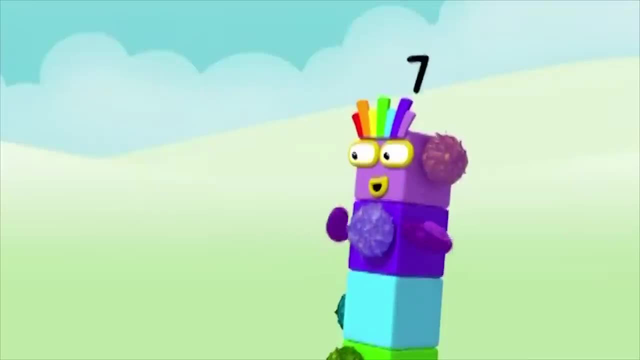 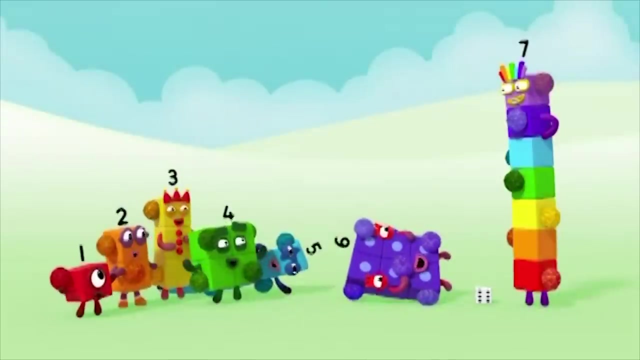 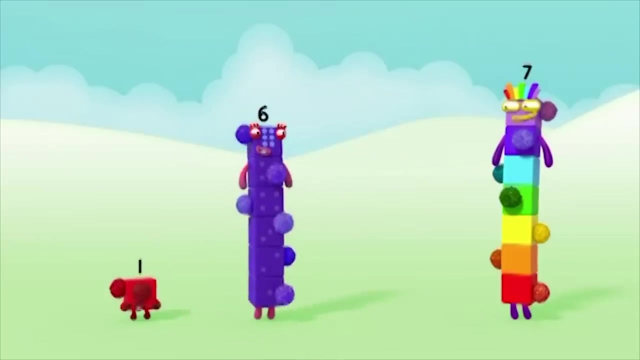 Of course I did. Sevens are not ticklish. How lucky is that. Oh, have you all had enough tickling? Why don't you just make sevens? then How? I'll show you One and six. One plus six equals seven. 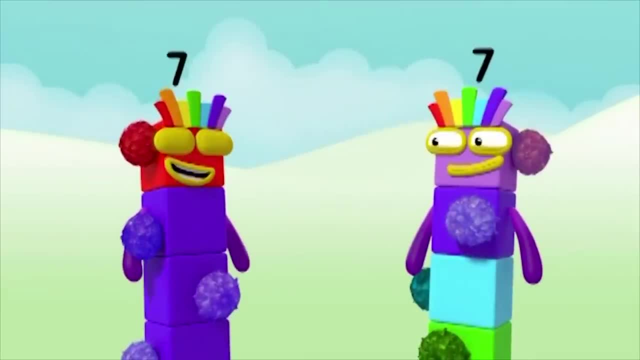 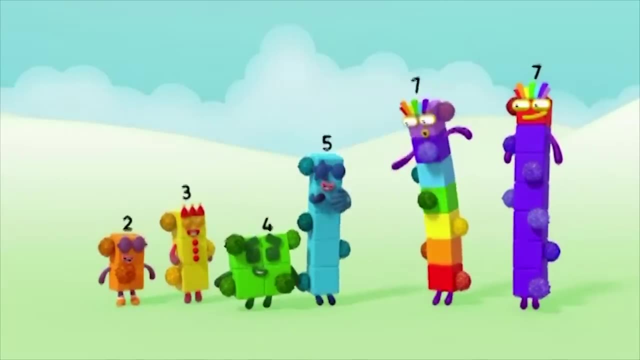 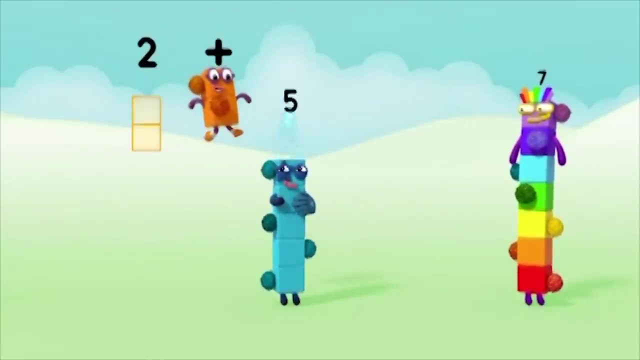 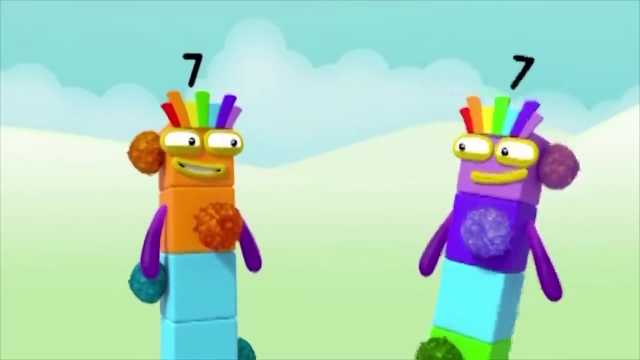 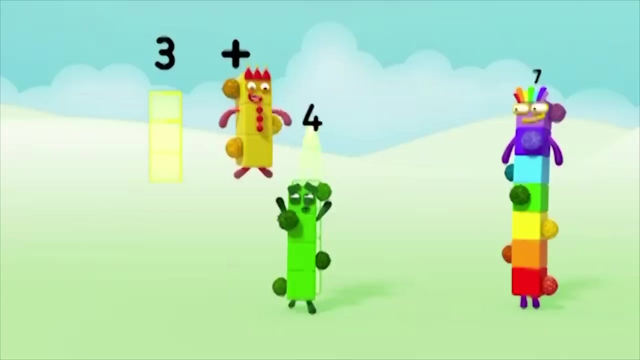 Seven. One plus six equals strong. One plus six equals strong. Oh, that's better. Pick me Blue. Two and five. Two plus five equals seven. Oh, that's better. Three and four: No, Oh, they've all stopped. 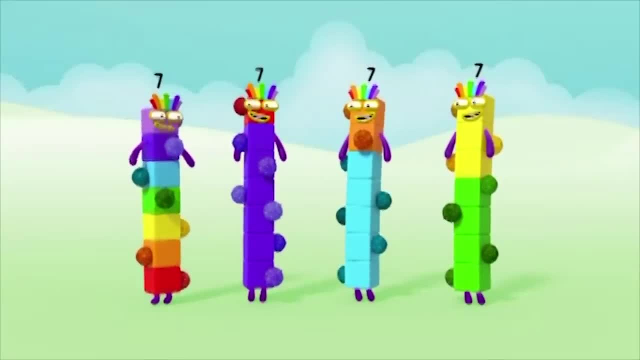 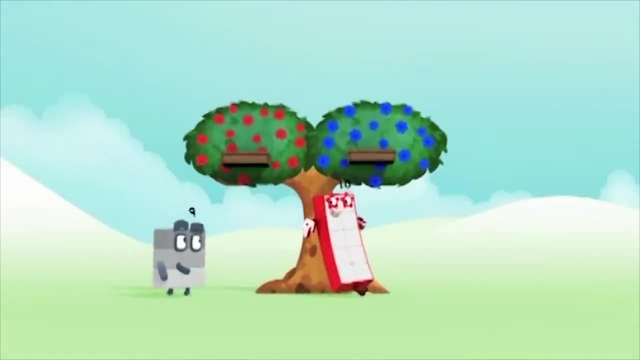 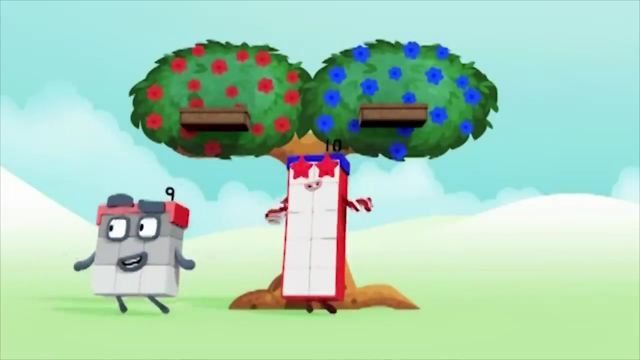 We're so lucky Fancy. a game of throwing twos- You be reds, I'll be blues- Sounds like fun. I'll draw a line. I'm bigger, so I'll start. Ten Minus ten Equals eight. 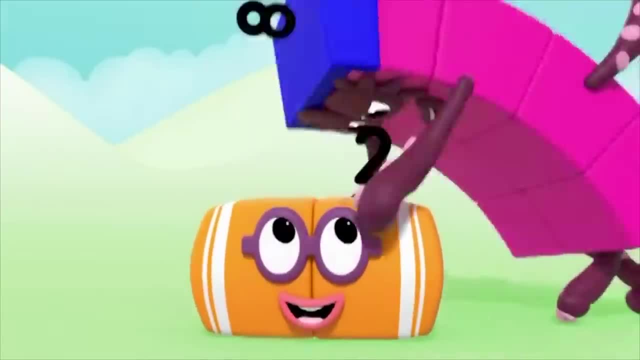 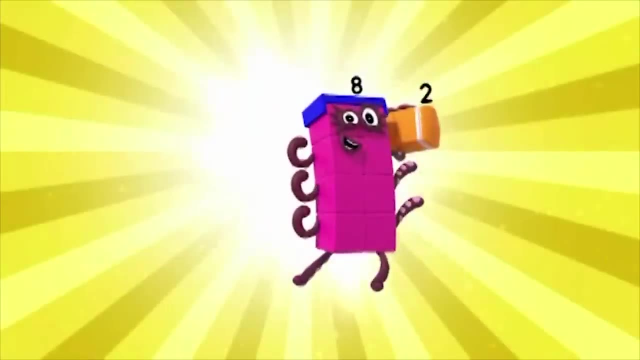 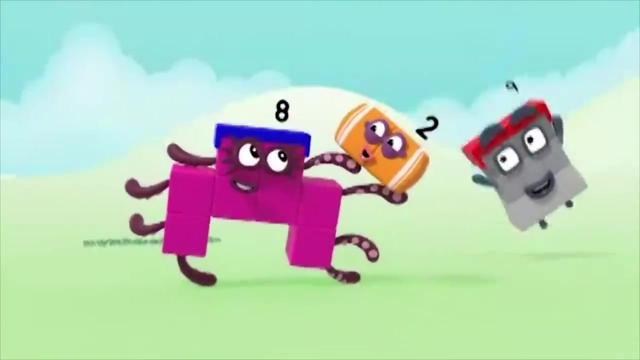 Game on: Ready go, Octoblock. play One, two, three, four, five, six, seven, eight play. He's on the left And now the right. He's on my head now, out of sight. 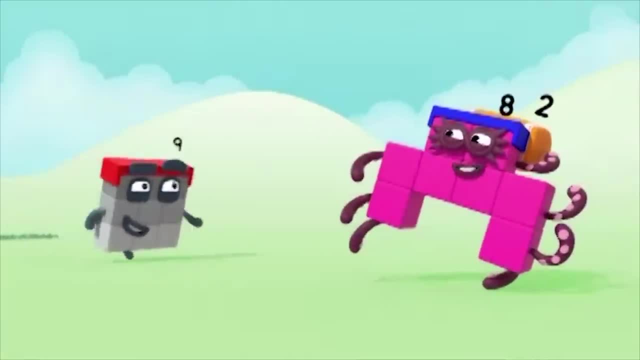 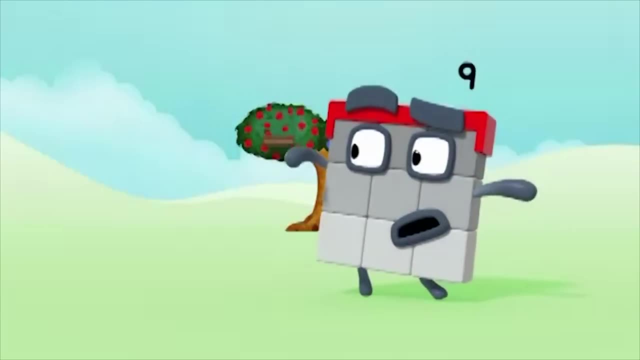 Woo-hoo, I'm going to get you Octoblock. I'm going to get you Octoblock Up high, down low, too slow, Ah-ah-ah-ah-ah, Achoo Whee. 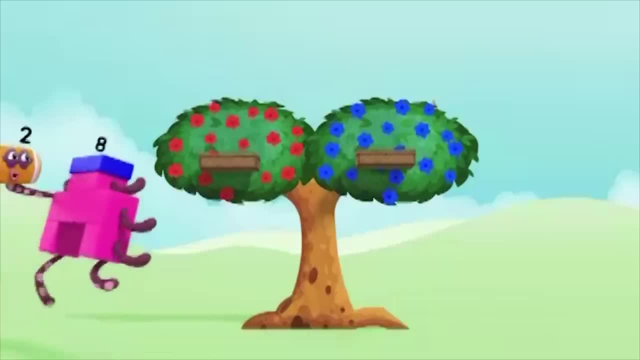 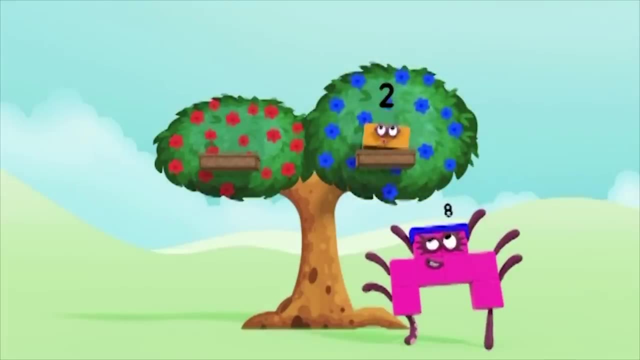 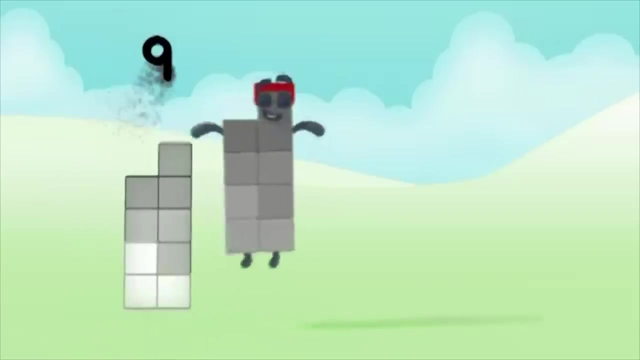 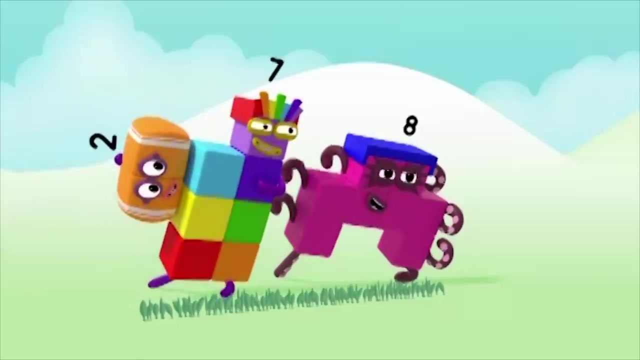 Huh, Octoblock, jump, Woo-hoo. Score Two points to blues. I'm bigger now, so it's my turn. Nine Minus Minus two Equals seven. Ready Go, Huh, Uh. 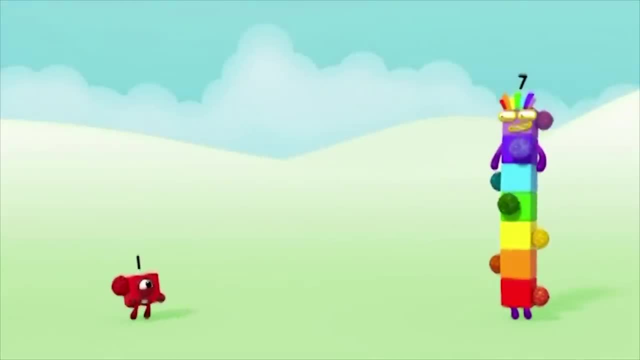 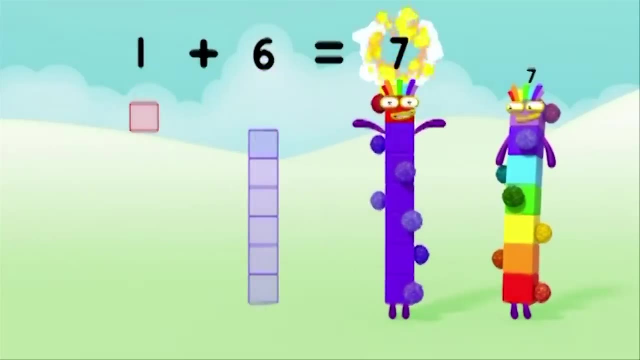 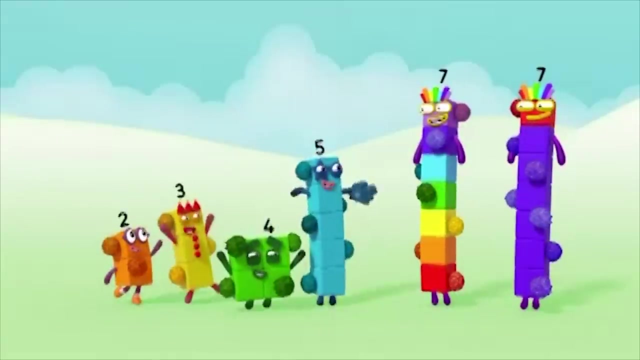 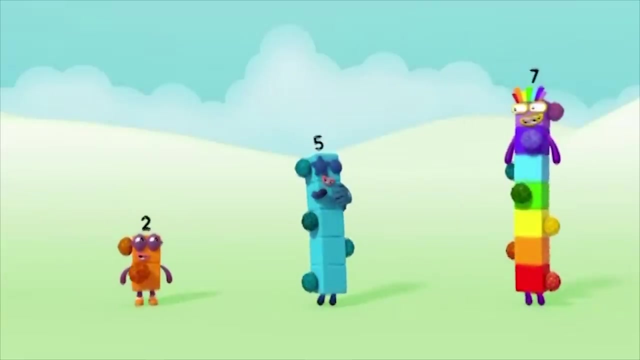 I'll show you One and six. One plus six equals Sevens, Sevens, Sevens, Oh, that's better. Pick me Three, Two and five. Two plus five equals seven. Two plus five equals seven. That's better. Three and four, Three and four. 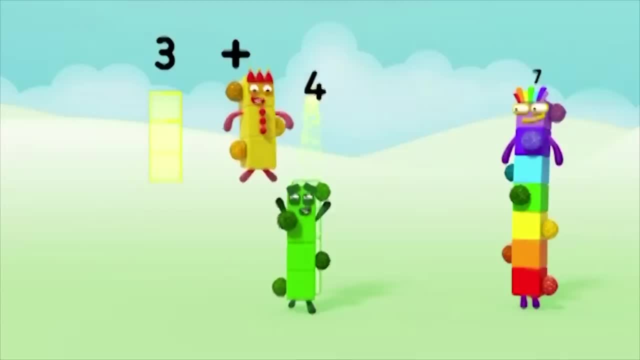 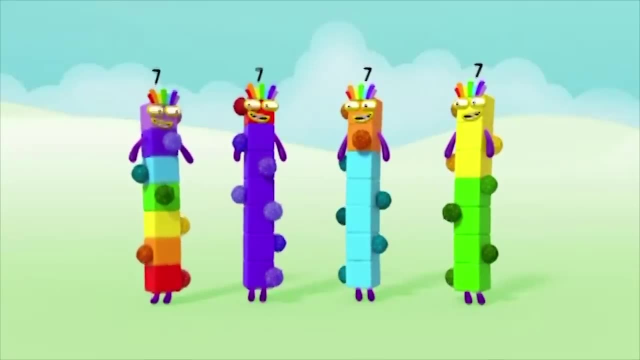 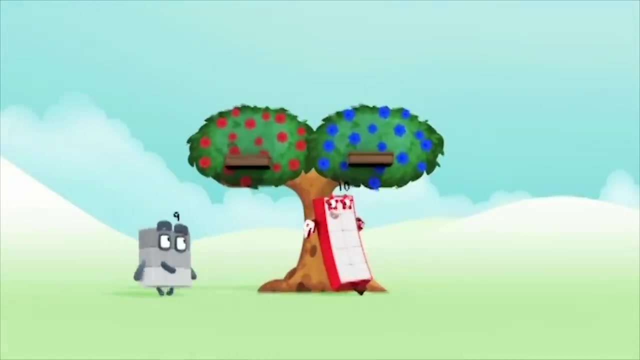 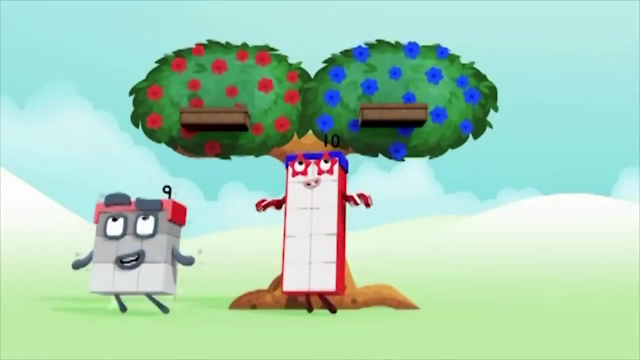 Three and four. Three Plus four equals seven. Ah, they've all stopped. We're so lucky. Fancy a game of throwing twos. You be reds, I'll be blues. Sounds like fun. I'll draw a line. I'm bigger, so I'll start. 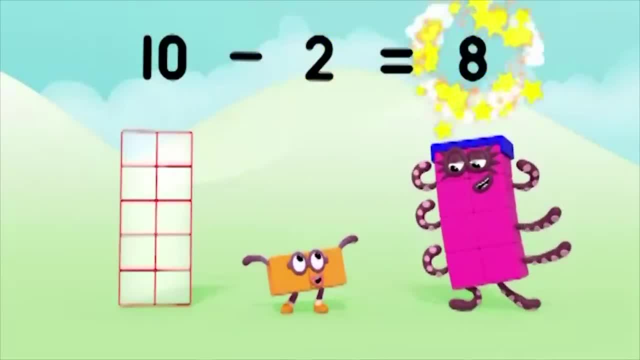 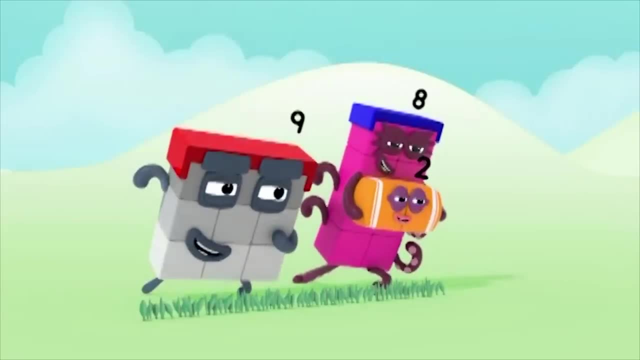 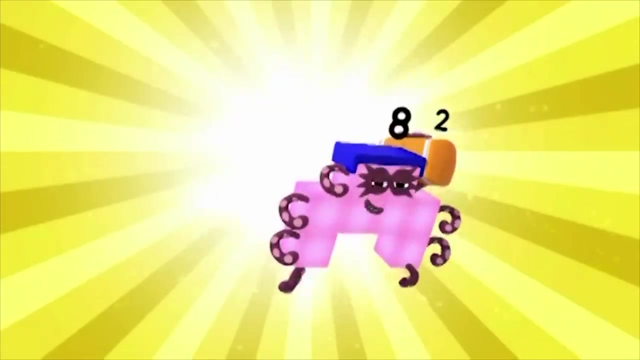 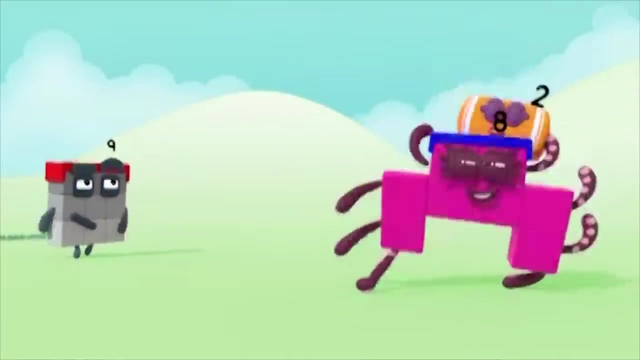 Ten minus two Equals eight. Game on: Ready go Up to block. play One, two, three, four, five, six, seven, eight play. He's on the left And now the right. He's on my head now out of sight. 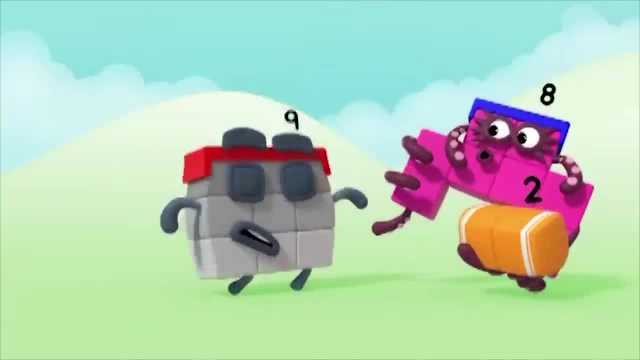 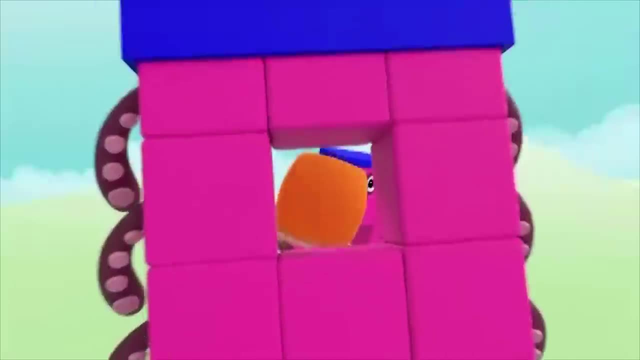 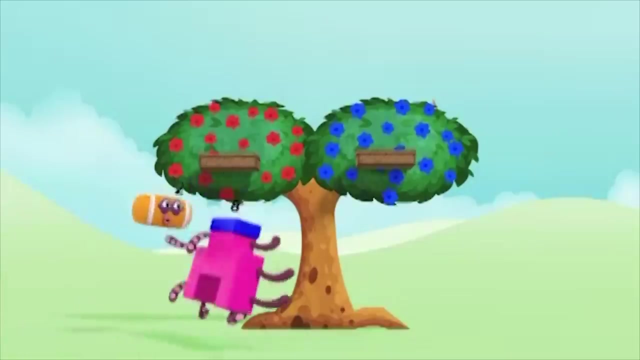 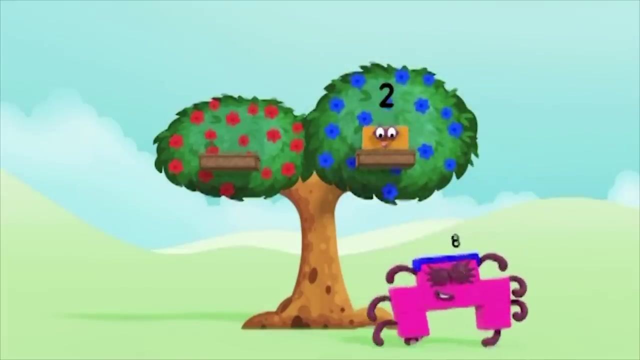 Woo-hoo Up high, Down low, Too slow. Ha-ha-ha-ha, Achoo Whee Huh, Up to block jump. Woo-hoo, Score Two points to blues. I'm bigger now, so it's my turn. 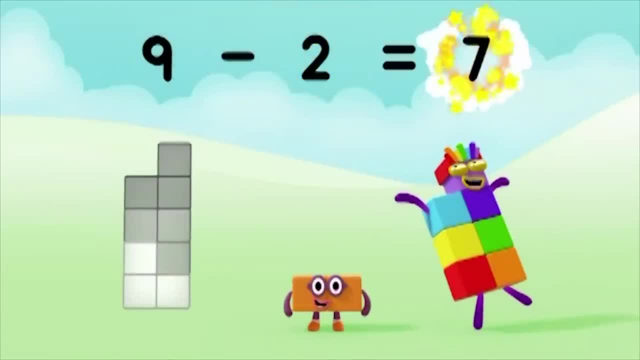 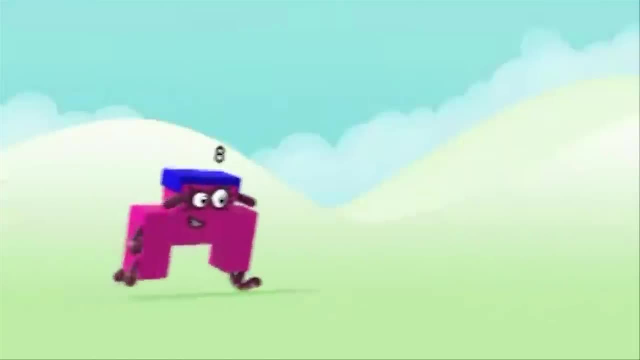 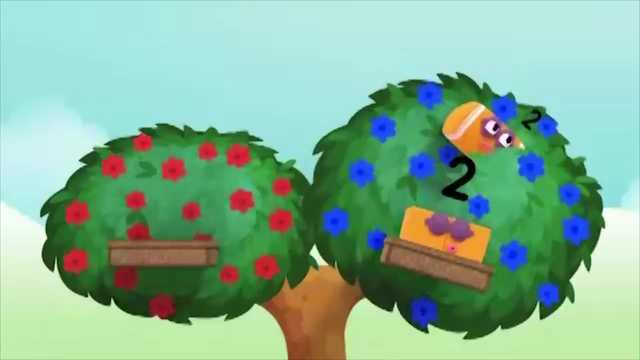 Nine minus two equals Seven. Seven Ready Go? Huh, Uh, Whee, Woo, Woo-hoo Whee. Two points each. Beginner's luck, You're bigger, You start Eight Minus two. 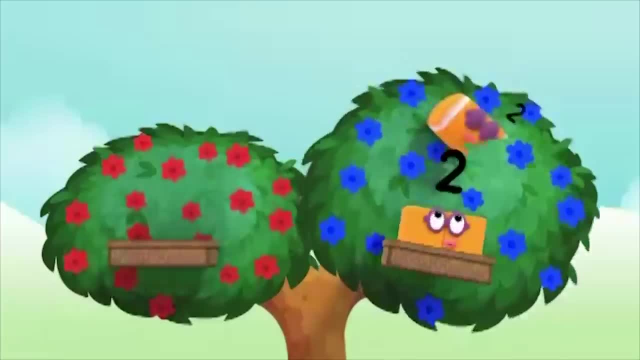 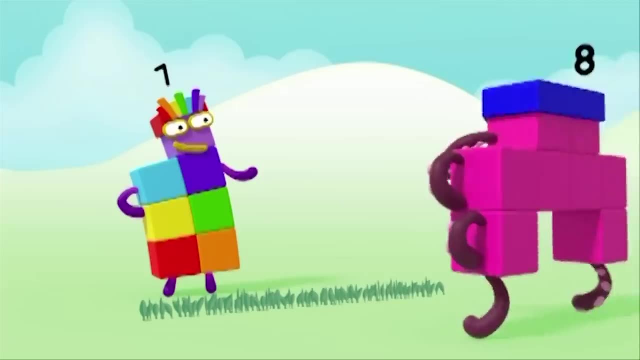 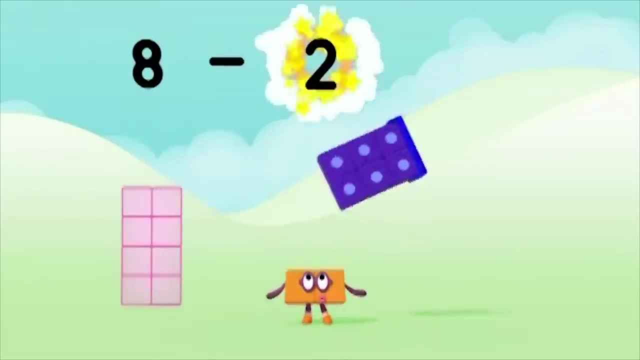 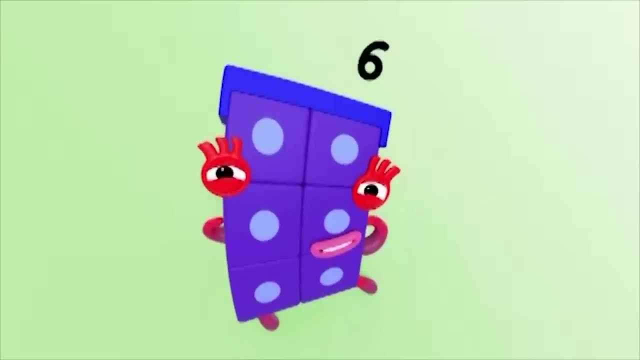 Whee, Woo-hoo-hoo-hoo. Oh Whee, Two points each. Beginner's luck, You're bigger, you start. Eight Minus two Equals six. Whee, Whee, Whee, Whee. 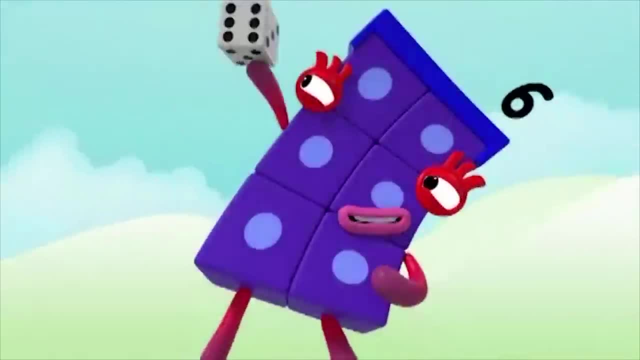 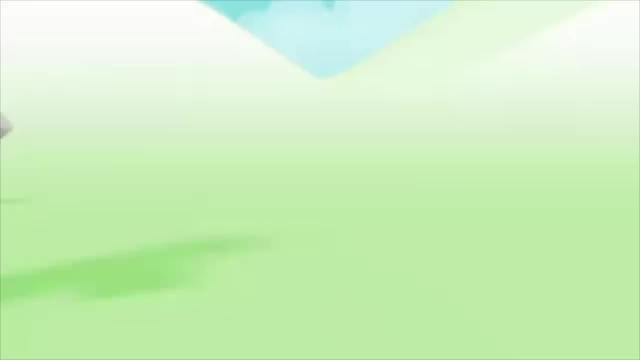 Whee, This game is nice. Let's roll the dice. When it leaves my hand, how will it land Um On six? Ooh Ha Ha. Oh, Lucky me, Ha-ha-ha, Lucky me. 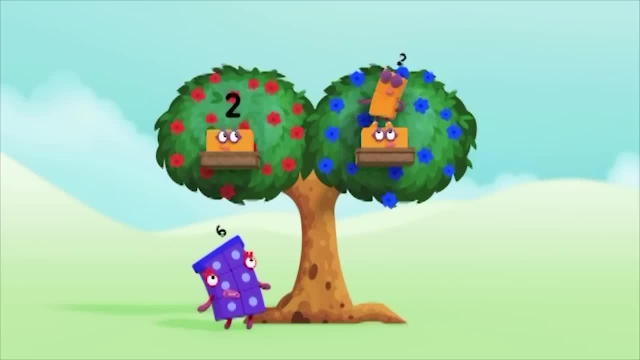 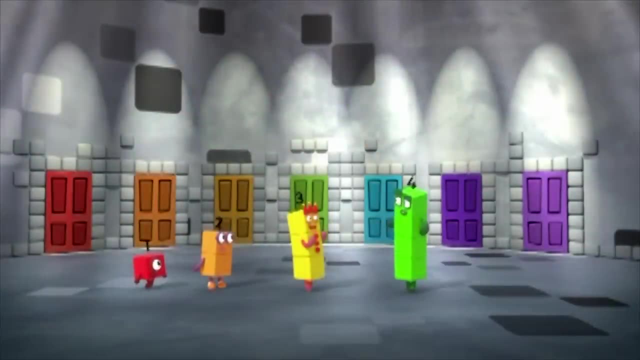 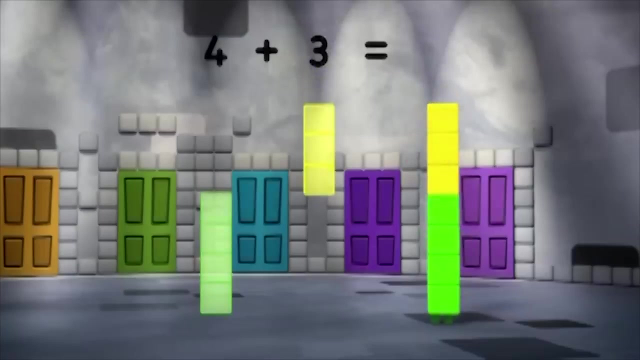 Woo-hoo, Penalty, unfair distraction, Which means Four, two, Seven doors. Which door is right? Maybe seven can help. How do we get seven? Four Plus three Equals Seven. Ooh, I feel lucky. 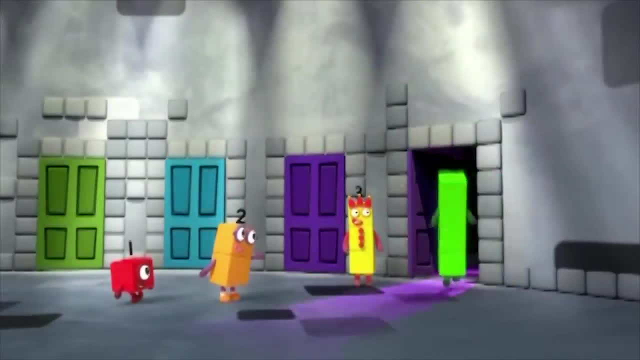 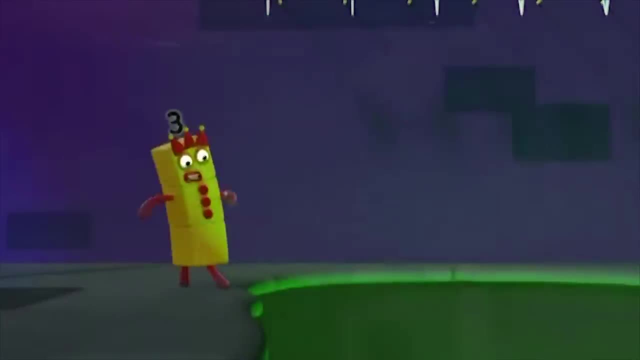 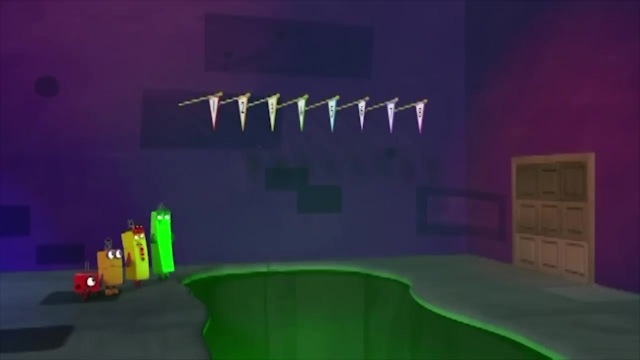 Whoa, This way, Easy-peasy, look-a-measy. Oh, We're stuck. No, we're not. We could swing from the flagpoles. We'd need someone with very long arms to stretch that high. Eight, How do we get eight? 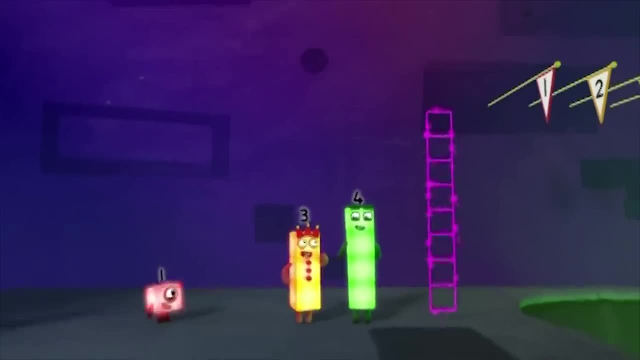 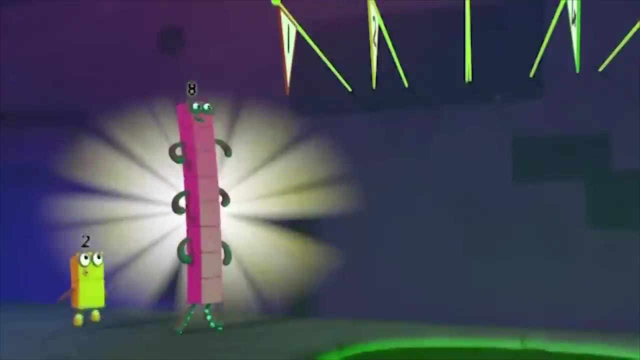 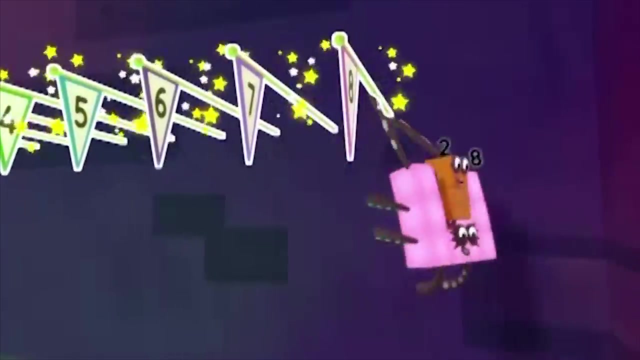 Oh yeah, Hmm, Four Plus three Plus one Equals Eight Octoblocks, Octoblocks, Swing Whee. One, two, three, four, five, six, seven, eight, Swing BANG. 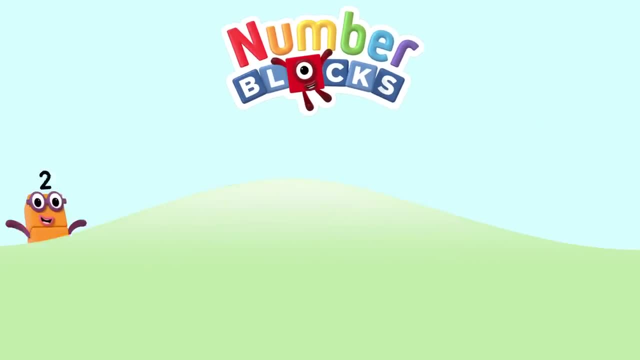 One, two, three, four, five. number blocks One, two, three, four, five. number blocks One and another, one is two and another one is Me, That's three, five, four, three, two, one. 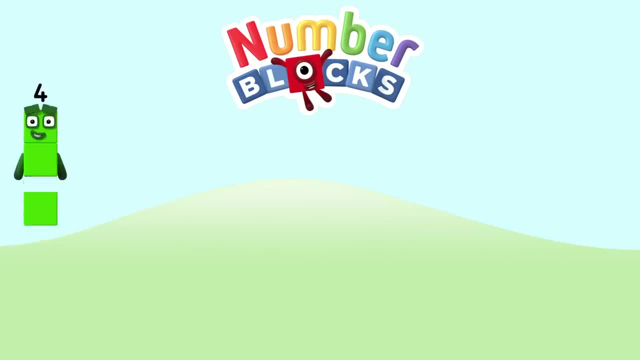 Time for some number fun. You can count on us with a number box. Subtitles by SteamTeamExtra.